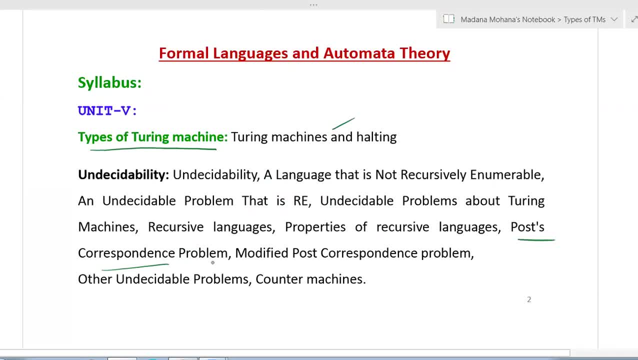 give some set of lists with set of integers. so whether these lists have post correspondence solution or not, they want to solve small problem. this is very interesting problem. then, modification of post correspondence. we have modified post correspondence problem. then we will see later some other undecidable problems. this counter mission also we will cover under one of the type. 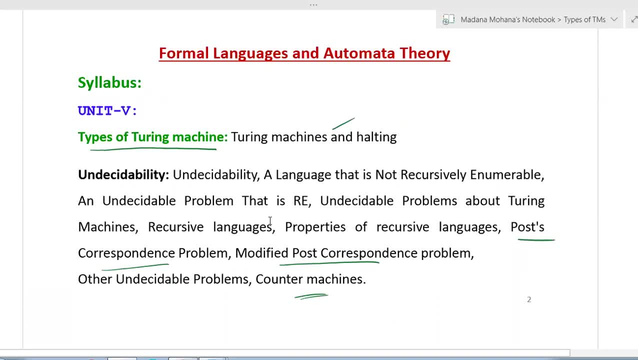 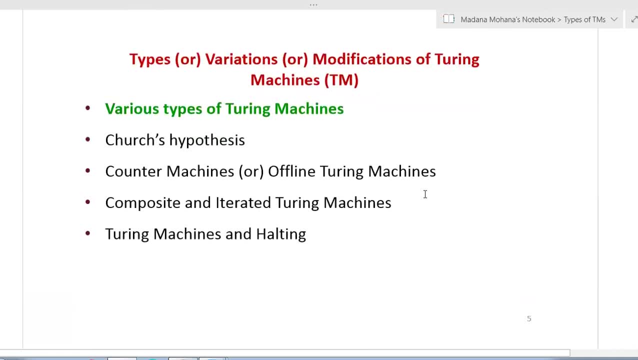 of turing mission. so now let us move to our actual topic. so here under types also called as variations or also called as modifications of turing mission. so in examination if you will get theory question, there may be chance of getting question on this. they will ask types of turing missions or 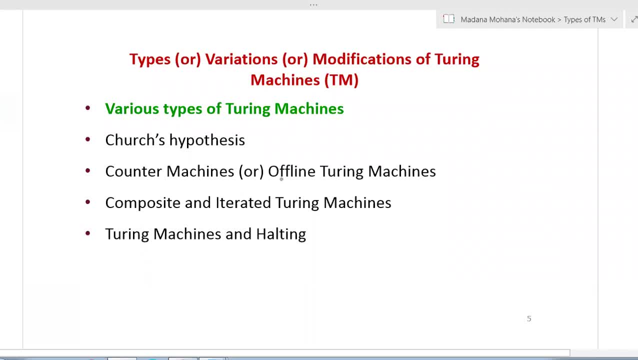 specifically some particular names are given. you can explain about so on. so type of turing mission or these concepts, also somewhat important. if you will get some short answers type or uh, b, c, like so chet's hypothesis, that also will cover very small topic. then counter mission or offline turing mission: this is also one kind of turing mission. 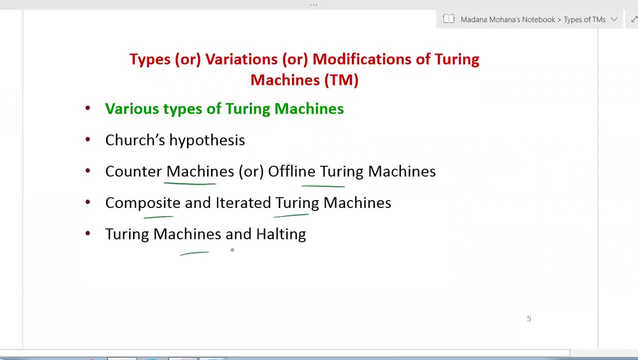 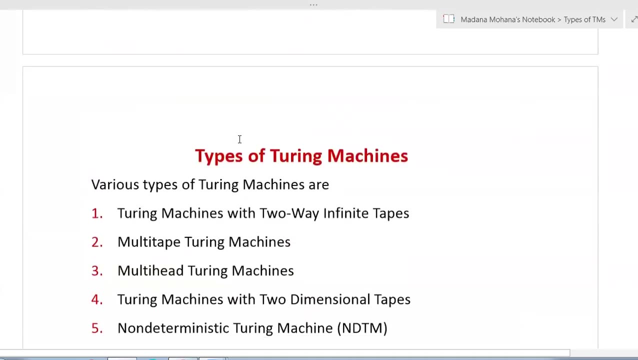 then composite and iterated turing mission, then turing mission and halting. so all these, whatever the topics we are going to cover, broadly comes under the category of types or variations or modifications of turing mission. now let us see the first category: types of turing missions. 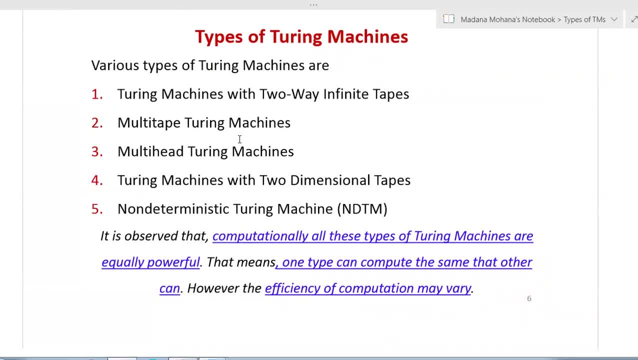 so majorly, various types of turing missions are given below. the first one is turing mission with two-way infinite tape. but all these types, the base model is same as our basic turing mission with some modifications, with some enhancements. you will get various types of turing missions. the first one is turing missions. 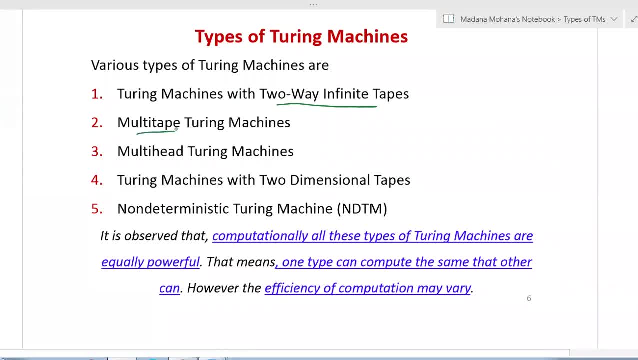 with two-way infinite tape, then the second one is multi-tape turing mission, then third one is multi-head turing mission, then the fourth one is turing mission with the two-dimensional tape, then fifth one is non-deterministic turing mission. so here you can observe the name itself clearly. 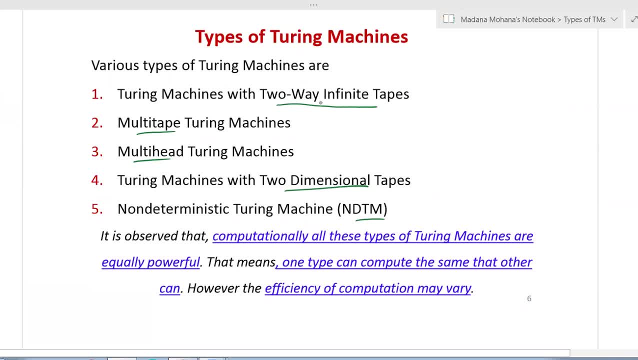 gives the variation: first turing mission with two-way infinite tape. anyway, the turing tape is infinite, but both ways it has to be extended infinitely. then that is called as two-way infinite tape, then multi-tape turing mission. here you can see the name itself, multi-tape. 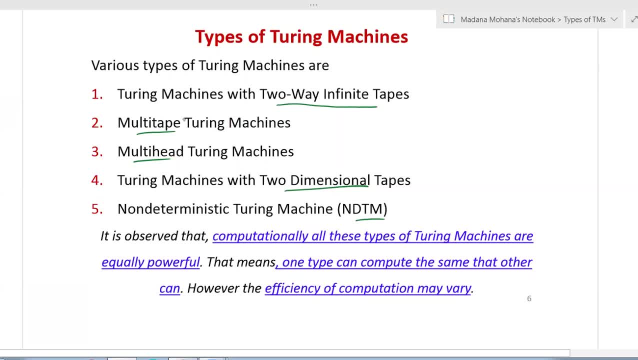 more than one type. in the basic model of turing mission we have only one type. but if it contains more than one type then that is called as multi-type turing mission. then multi-head turing mission means with the basic model with one turing mission more than one read or write header. then 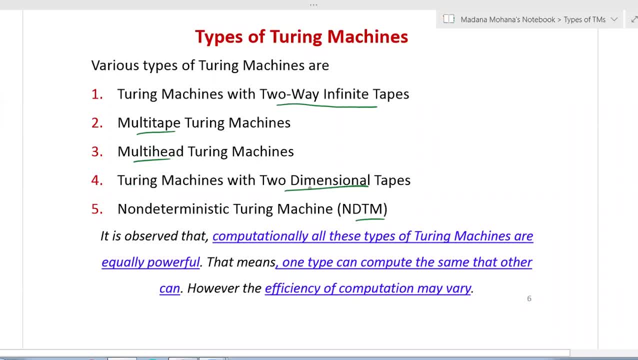 that is called as multi-head turing mission, then turing missions with two-dimensional tape. so normally we will consider our turing mission with one one-dimensional, one-dimensional tape only. so whenever the dimensionality is increased, one-dimensional to two-dimensional or more than two, then there is multi-dimensional, then the turing mission is called: 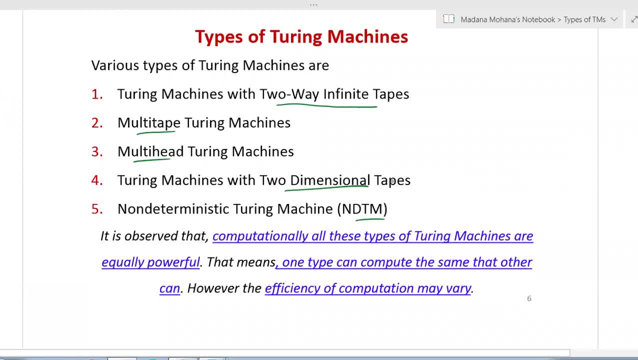 as turing mission with two-dimensional, multi-dimensional tape only tape dimension is changed. then non-deterministic turing mission, then the concept of non-determinism we discussed in finite automaton, in pushdown automaton also, then in turing mission also. so this is simplified. 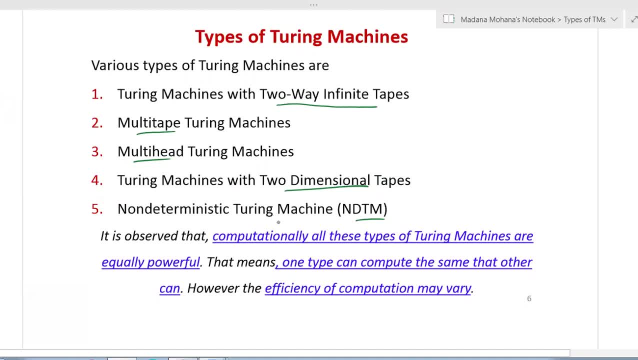 to non-deterministic, finite automaton. why? because turing mission is essentially a finite automaton. so here you know. you can observe one commonality among all these types: it is observed that, computationally, all these types of turing missions are equally powerful. the computational power of all. 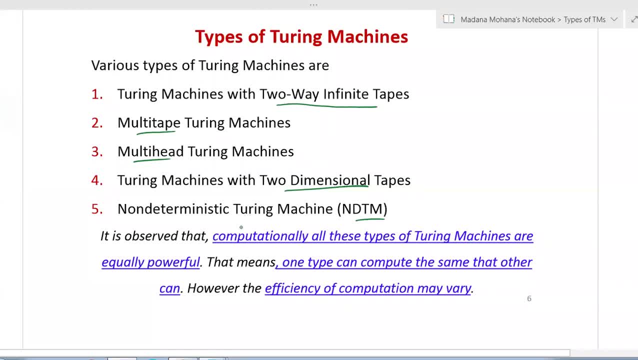 these types of turing missions have the same. that means one type can compute the same that other can do. but, however, where all these five are, differ with respect to efficiency of computation, so the efficiency of computation may vary one type to other type. so these are all the similarities and differences. 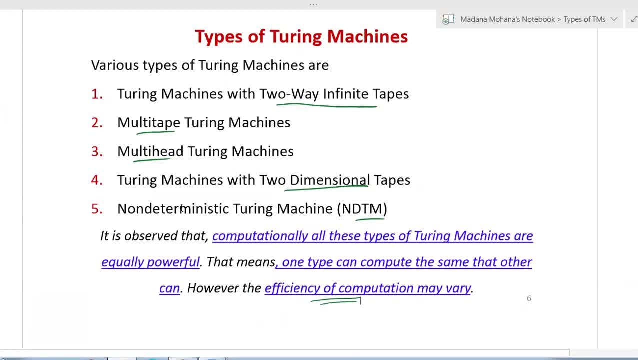 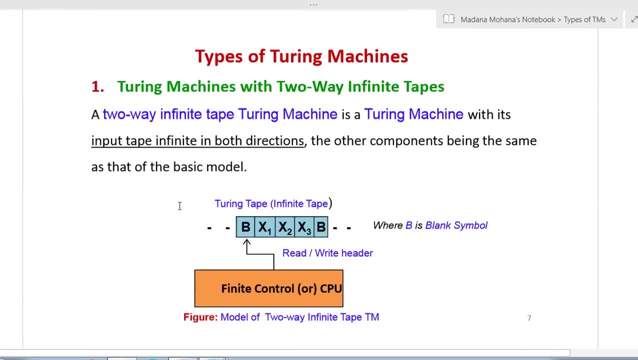 among various types of turing missions. now we will see one by one turing mission with the diagrammatic representation followed by some description. so the first one, turing mission with two-way infinite tape. so here you can observe, this looks like our basic model of turing mission only. but the only thing is that turing tape should 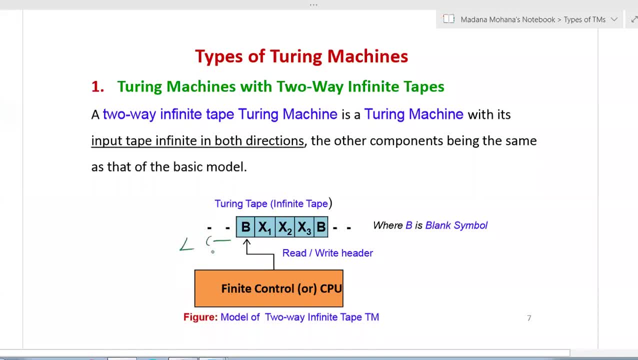 be extended in both directions infinitely towards left and towards right. but in the basic model also we have taken same diagram only. but in the model of turing mission. there we restricted the left hand, then right hand is open to extend infinitely. so here a two-way infinite tape. turing mission is a 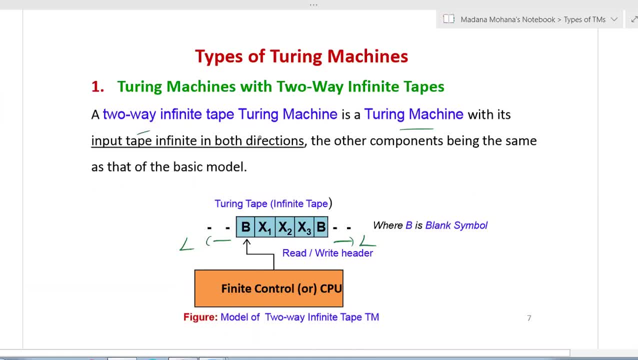 turing mission with its input tape, infinite in both directions. so that is left and right, the other components being the same as that of the basic model. then the operation. so all the components, description, everything is safe. so here the tape is extended towards left hand by including blank symbol. then 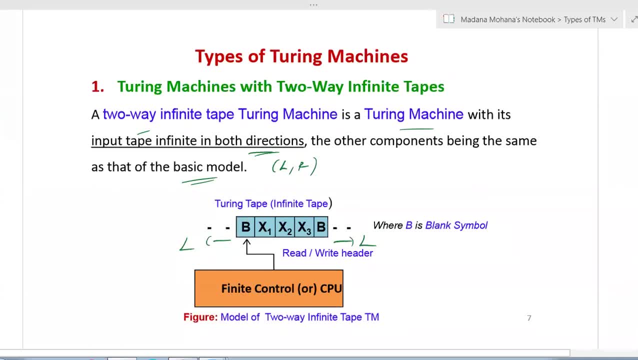 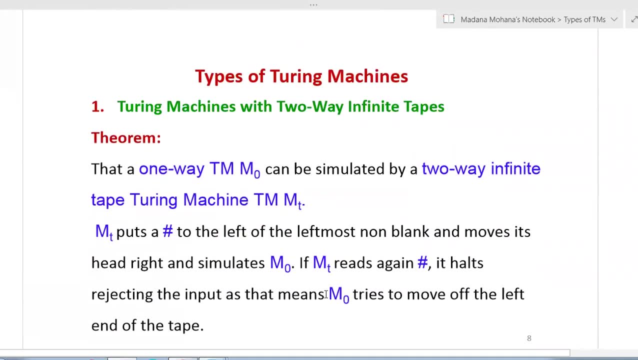 towards right hand by including blank symbols. this is a model of turing mission with two-way infinite tape. then some words: right hand, by including blank symbols. this is the model of turing mission with a two-way, infinite tape. then some aspects about this two-way, infinitive turing mission. here we have one theorem. So whenever 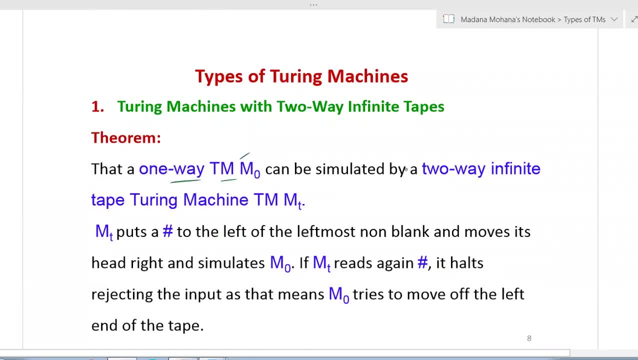 we have one-way turing mission, let us say m naught can be simulated by a two-way infinite turing mission. t m, let us say m t. that means, whenever we have one-way turing mission, that is our basic turing mission. so then that can be simulated by a two-way infinite runtime. 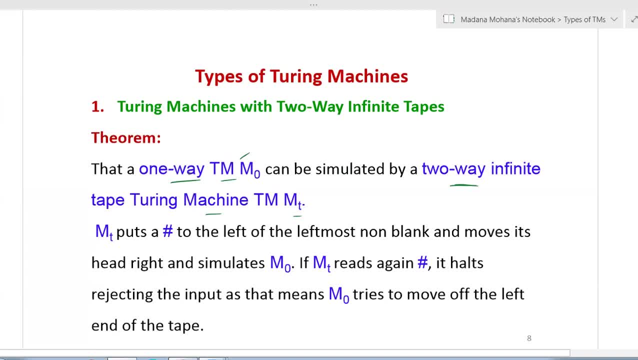 turing machine, let us say mt. so this is one theorem that is equivalence of one way to two way infinitive turing machine. so here, mt, that is, the two-way infinitive turing machine, puts a hash symbol, which is called as the end marker, to the left of the leftmost non-blank and moves. 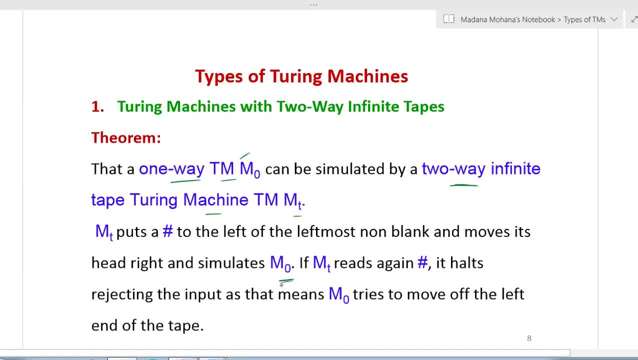 it head right and simulates m0. that is one way infinitive turing machine, even in finite atom. also the movement of read right head will be in left direction and right direction, but that is restricted towards right only by keeping the end markers. one is at left hand and another one is at. 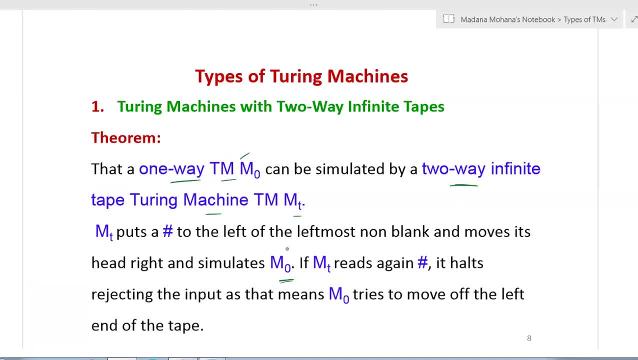 right hand, but then in the turing machine we are restricting the left hand by keeping the hash symbol that right hand is open. so then, if mt- that is the two-way infinitive turing machine- reads again a hash symbol, then it halts rejecting the input, as that means m0 tries to move off the left end of the tape. 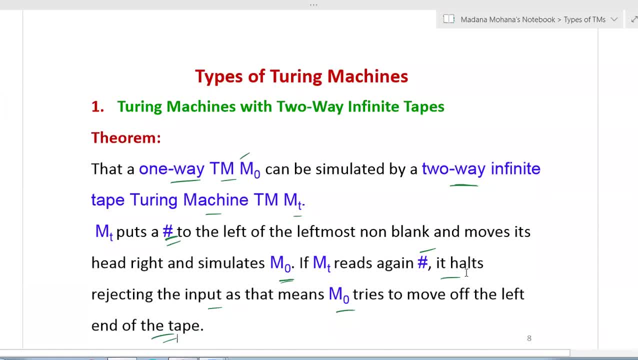 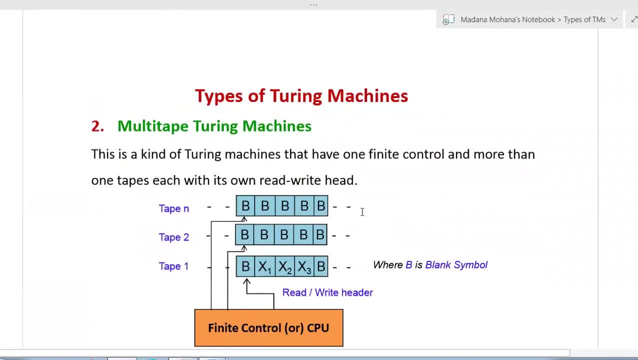 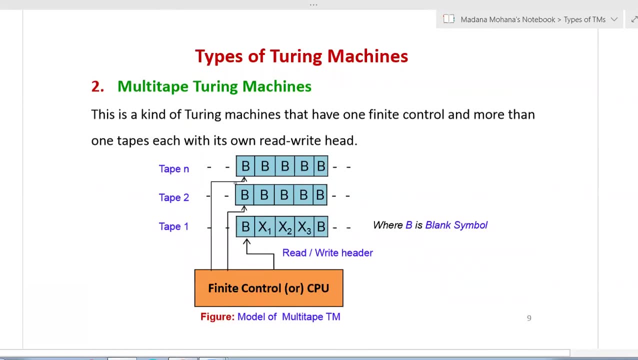 so whenever the end marker find, then mt halts by rejecting the input. so this is one theorem, followed by with some explanation. so now here move to the second type of turing machine, which is called as multi turing machine turing machine. here you can see the name itself gives so only. 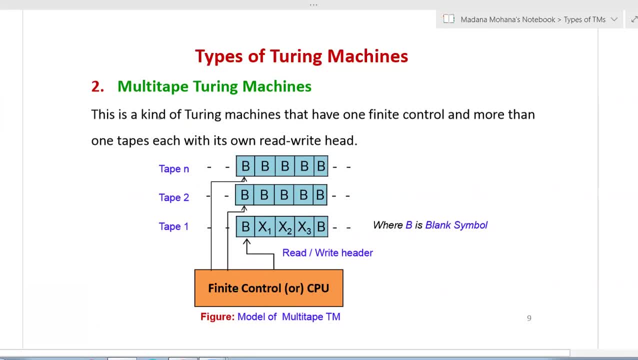 instead of one tape, here more than one tape is included, so that is called as multi-tape. if you can see the diagram, this is the model of multi-tape turing machine. only one, finite control. then see, here we have tape one, tape two, and so on. n tapes are there. so whenever we have 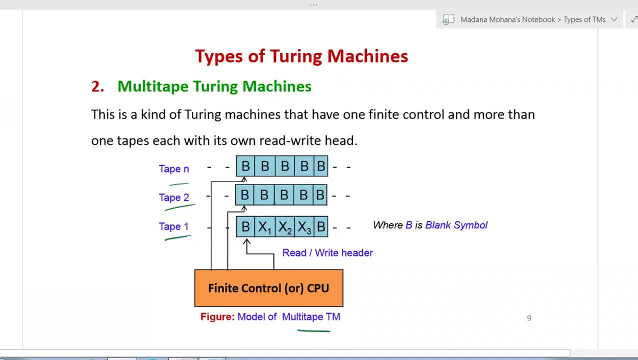 multi tapes are there. automatically, then for each tape one separate read write header is included. now you can see: for tape one, this is one read write header. then for tape two: this is read write header, then, and so on tape and this is reads write header. separate reader right headers. so now, here you can. 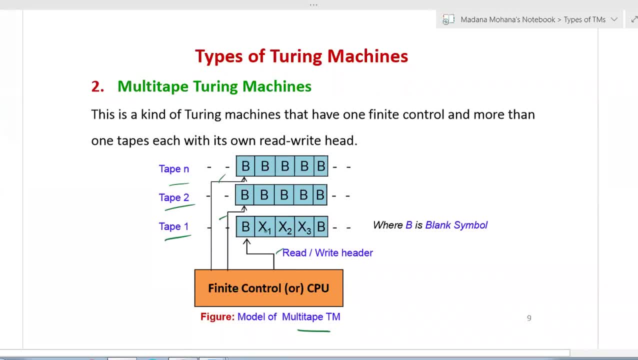 observe in multi tape turing machine, except the primary tape remaining all are stored with blank symbol. then the primary tape or tape one stores thelooked read write header breadingbelong input symbols, followed by blank symbols towards left and right hand. so now see, this is kind of. 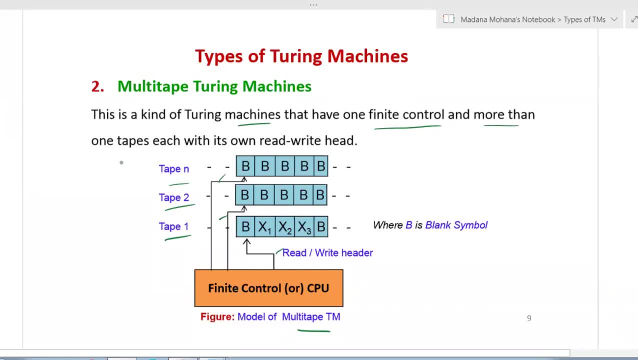 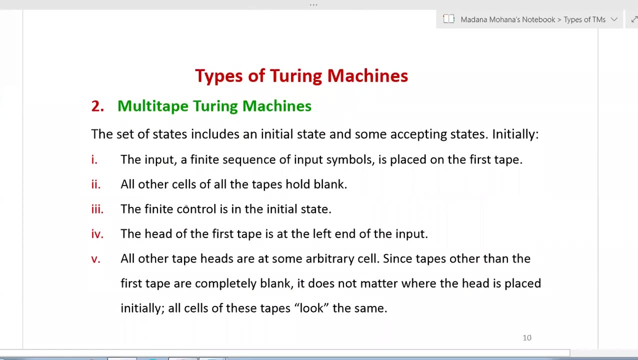 turing machine that have one finite control and more than one tape, each with its own read or write header. so this is a model or block diagram of multi-tape turing machine. now we can see some points related to this multi-tape turing machine. so the set of states includes an initial. 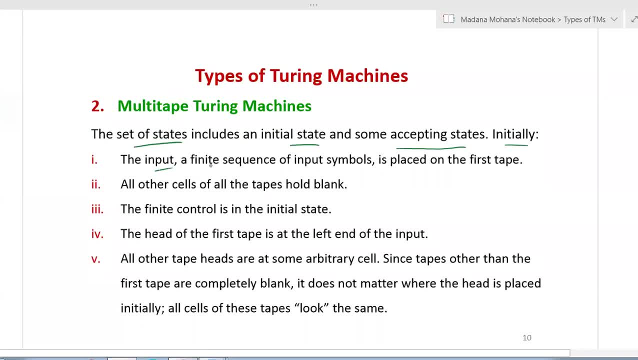 state and some accepting state. initially the input, a finite sequence of input symbols is placed on the first tape. just now we mentioned. all other cells of all tapes hold blank symbol. then the finite control is in the initial state. by default. the head of the first tape is at the 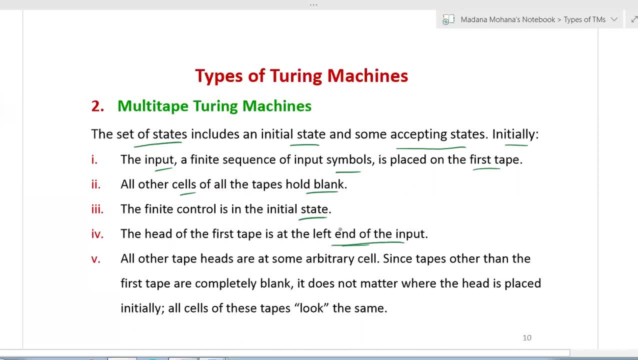 left end of the input. that means leftmost input symbol, where it is stored. then all other tape heads are at some arbitrary cell, not at the left end of the input. that means leftmost input symbol, where it is stored. then all other tape heads are at some arbitrary cell, not at the left end of the input. that means leftmost. 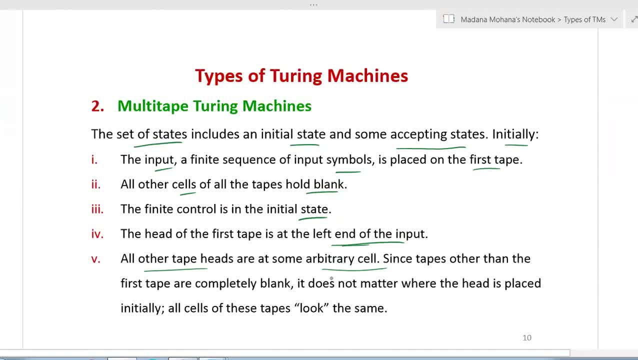 cell. only in the first tape reader header will be placed at the leftmost cell. then all other tape heads are at some arbitrary cell. since tapes other than the first tape are completely contains blank symbols, that means it doesn't matter where the head is placed initially. all 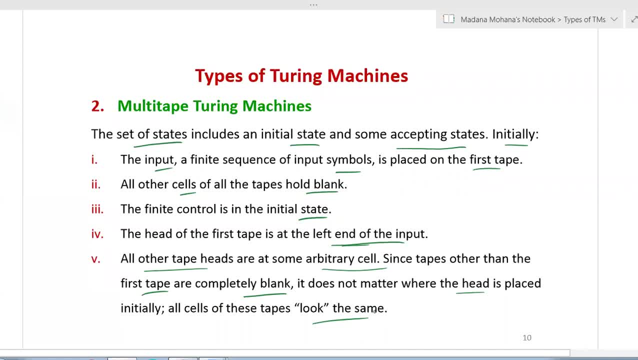 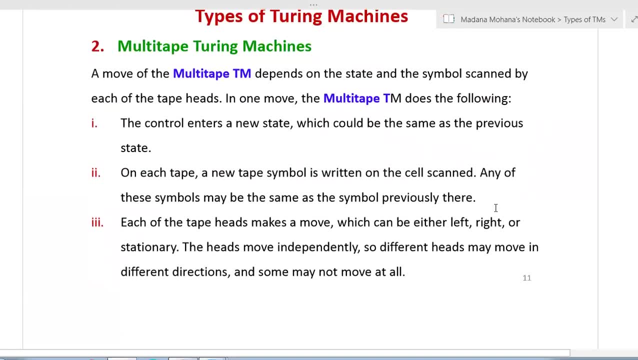 cells of these states look the same, other than the first tape. so these are some of the aspects initially, then then while considering the moves or transitions in multi-tapeturing mission, it depends on the state and the symbol scanned by each of the tape header. in one move, the multi-tapeturing mission does the 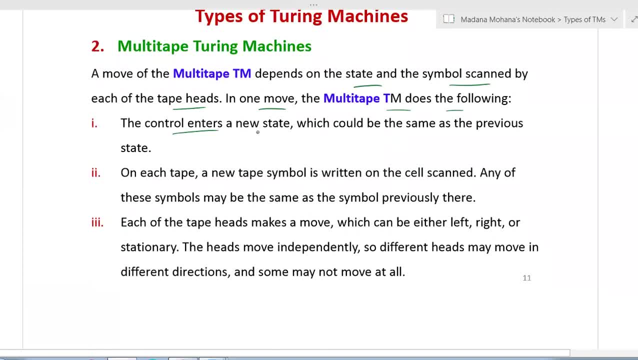 following first what it has to do. the control enters a new state which could be the same as the previous state. sometimes then on each tape a new tape symbol is written on the cell scanned. so whenever a cell is scanned then the new tape symbol is written on that cell. so any of these symbols may be same as. 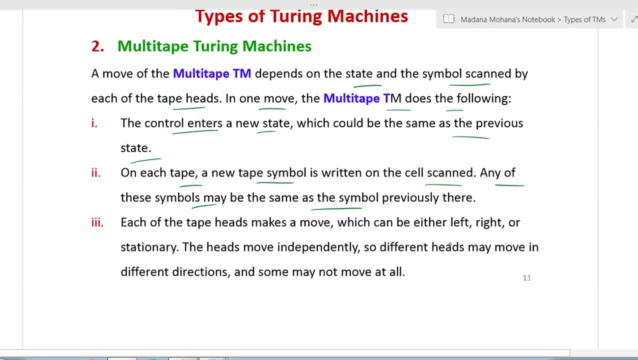 the symbols previously there in the design of turing vision we already seen, so sometimes we are skipping means. the same symbol is replaced with same, then it moves towards left or right, so that possibility is also there. then each of the tape head makes a move, which can be either: 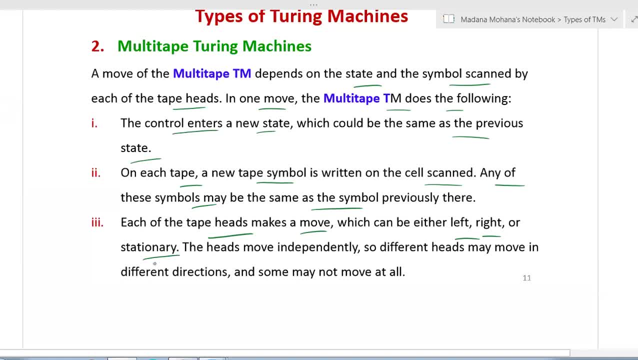 left, right or stationary. this is one more direction. stationary means no moment it will be in the same cell. the heads move independently, so different heads may move in different direction. there is no restriction on movement of read or write headers, one tape to other tape, and some may not move at all. that means yes. stationary, that means no movement. so in one move, in multi-tape. 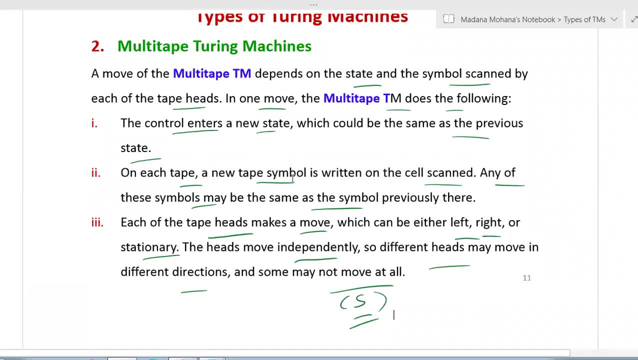 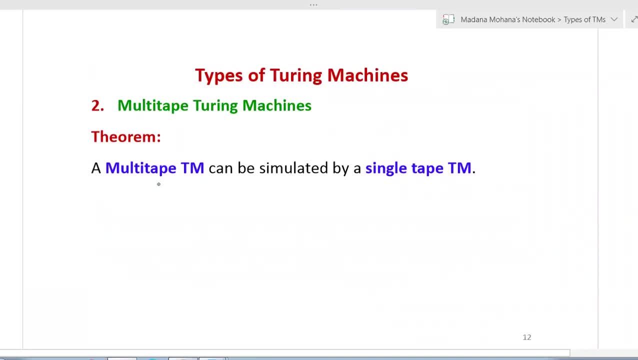 turing mission depends on the following aspects. then there is one theorem for multi-tape turing mission. so the theorem statement is: a multi-tape turing mission can be simulated by a single type turing mission, but reverse is not true here. then coming to the third type of touring mission, which is 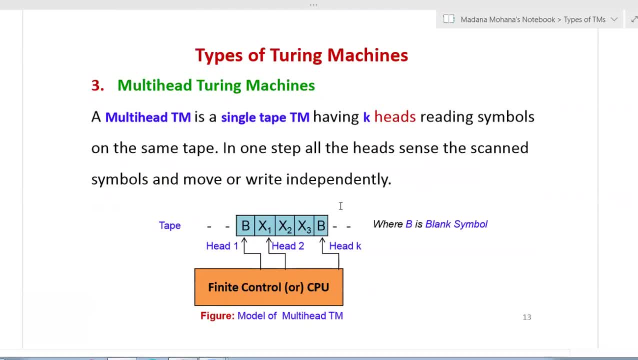 called as multi-head turing mission. here the name itself gives multi-head. that means with one turing tape, more than one head. so a multi-head turing mission is a single-type turing mission having k heads, reading symbols on the same tape, in one step all the 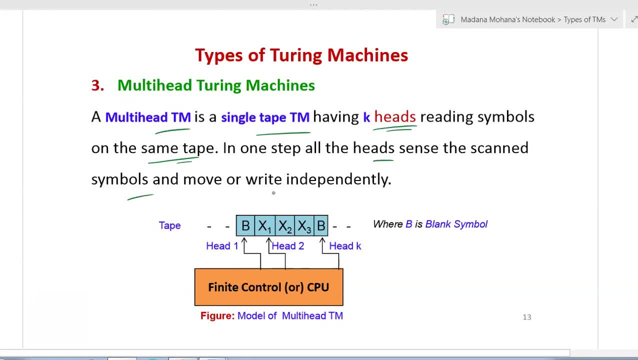 heads, sense the scanned symbols and move or write independently. now you can see the model or block diagram of multi-head turing machine. here see only one finite control, then one infinite turing tape. now you can see each input is scanned with one header. so now head one means read or write header. 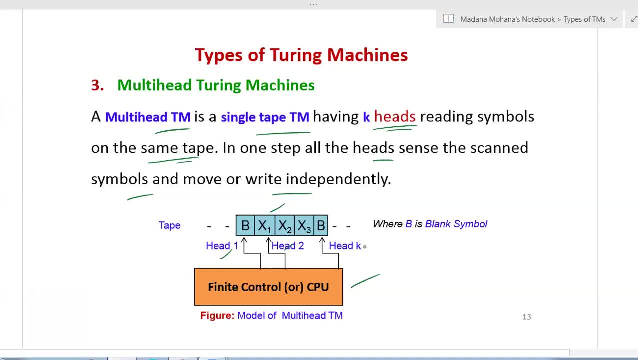 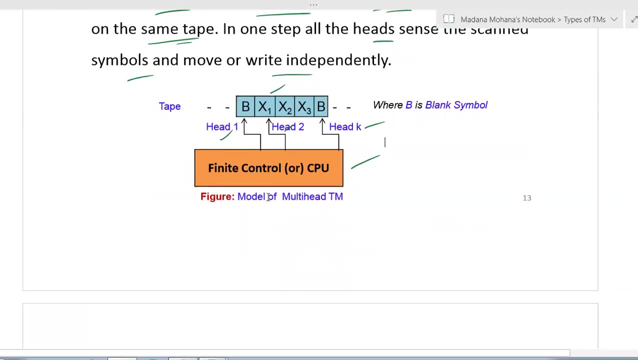 one, then read or write header two, and so on. read or write header. okay, so that is the multi-head turing machine. one tape, then multi heads. that means let us say k heads, then respective heads may read the respective positioned symbols. then it can be easily seen that these type of turing 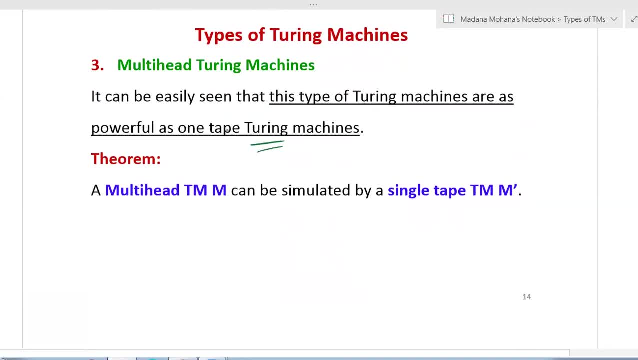 missions are as powerful as one type turing. which why? because at a time multi-tasking is performed here. now here also one theorem is there related to this one? a multi-head turing machine, m, can be simulated by a single type turing mission. let us say m. that then reverse, is not true here. 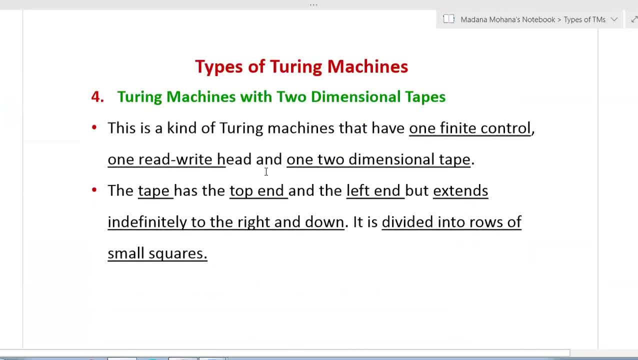 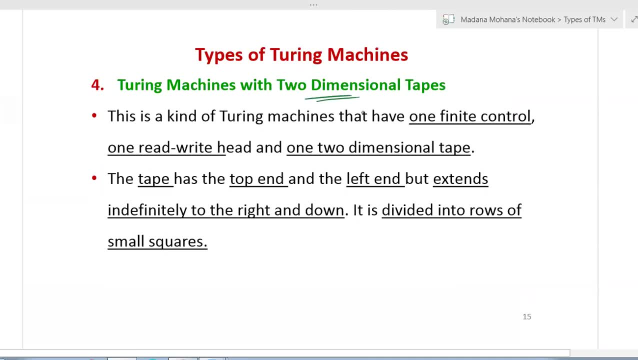 this is the theorem related to multi-head turing mission. then coming to fourth type of turing mission: turing missions with two dimensional tapes. that means more than one dimensional. here we will consider one example of two dimensional, then multi-dimensional, also more than two-dimensional. so this is a kind of turing mission that have one finite control, then one read. 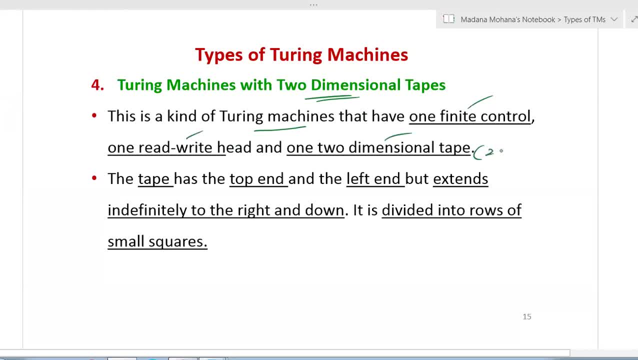 or right header, then one two-dimensional tape, that is 2d tape. the tape has the top end and the left end, but extends indefinitely to the right and down. also. here you can see: now the movement is top end, left end, then right and down. so here you can see, the movement is in four directions, so it is divided into rows of. 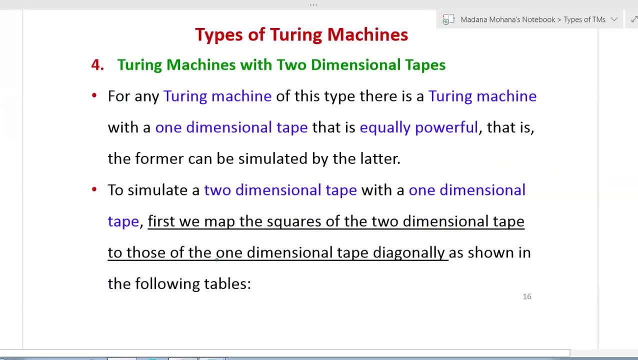 small squares. now this is generic for any turing mission of this type. there is a turing mission with one dimensional tape. that is our basic turing mission model. that is equally powerful, that is, the former can be simulated by the latter. that means two-dimensional. it is simulated with one dimensional, like, and so on. so to simulate a two-dimensional tape with a 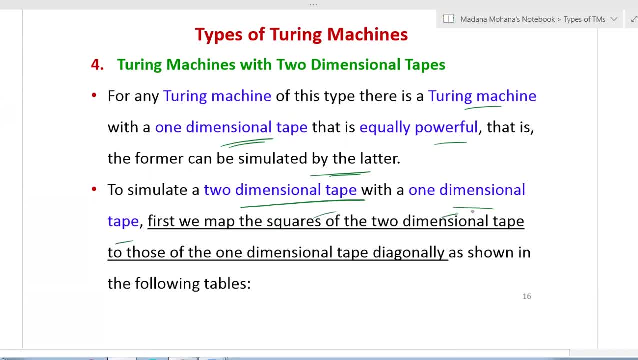 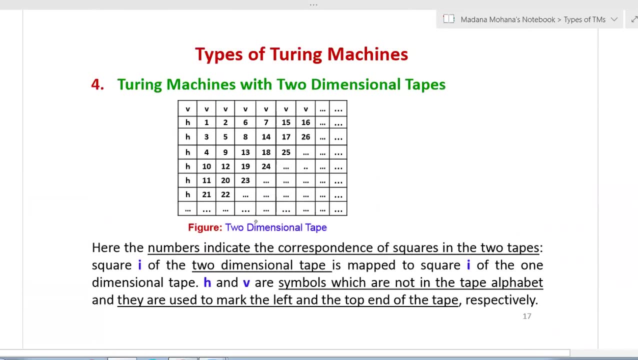 one-dimensional tape. first, what we have to do, we map the squares of the two-dimensional tape, those of one-dimensional tape, diagonally, as shown in the following table. so we'll consider diagonal mapping. now you can see, this diagram shows example of a two-dimensional tape. so which? 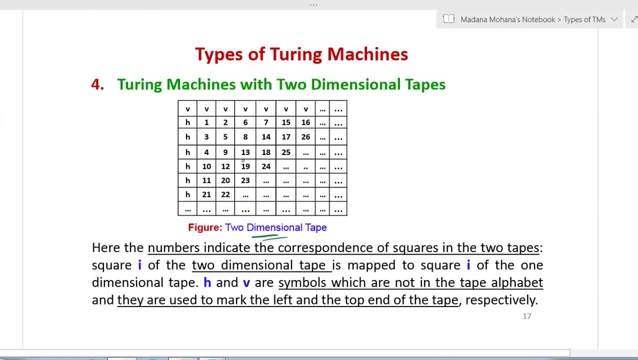 can be divided into cells with rows and column combinations. so here the row and column are added with some special symbols, like blank symbol. then all other rows and columns are filled with the values or symbols of the input, with diagonally. now you can see here the numbers indicate. 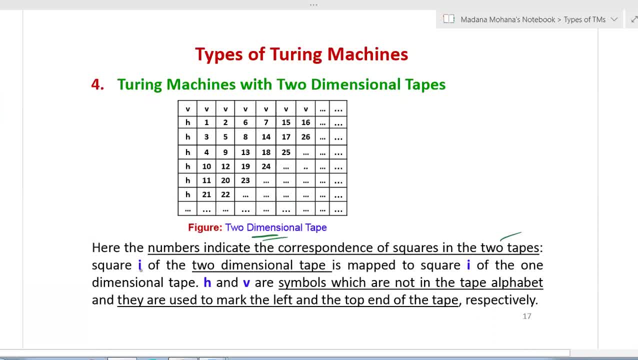 correspondence of squares in the two tapes. so for example, square i of the two-dimensional tape is mapped to square i of one-dimensional tape. so now the corresponding correspondence here in two-dimensional the corresponding square is i, then in one-dimensional the corresponding square is i. so this should be matched, matched similarly. suppose here we use: 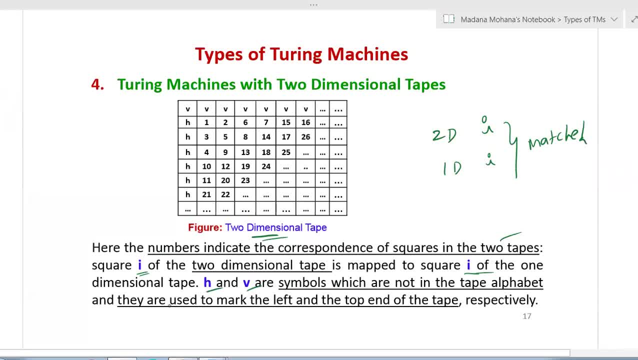 h and v are symbols which are not in tape alphabet and they are used to mark the left and the top end of the tape. so h is the left and v is the top end. here you can see: this is the left now. this is the top end. so this is left now. this is a top end. 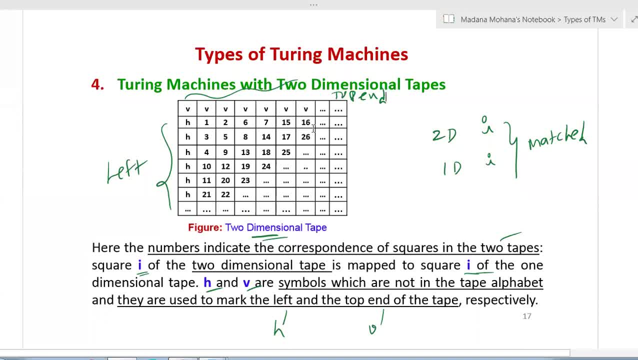 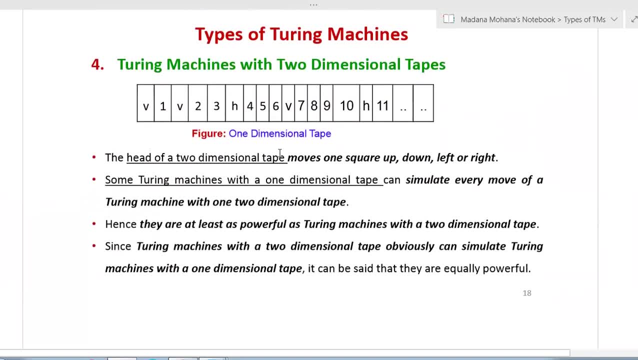 so respectively: this is the example of two-dimensional tape and the data how this can be stored. now you can see we will compare with the two-dimensional tape with one-dimensional tape. so this is the diagram which is example of one-dimensional type. one-dimensional tape means our normal basic model curing tape. so here you can observe, here the tape is divided. 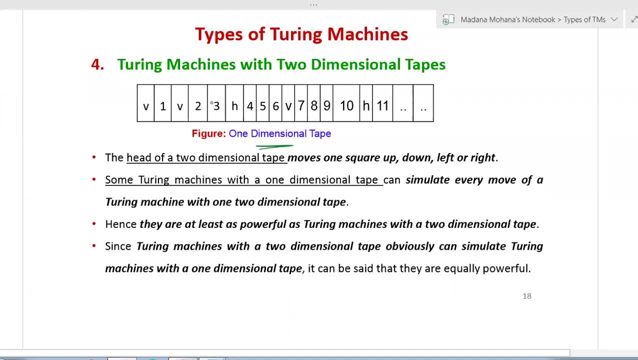 into number of cells. each cell holds one symbol at a time. then all the symbols are included with the combination of the previous values, v and h. also here, v and h combinations are there. why? because this has to match with two-dimensional tape. so the head of the two-dimensional tape moves one square up, one square down, one square left or one square right. 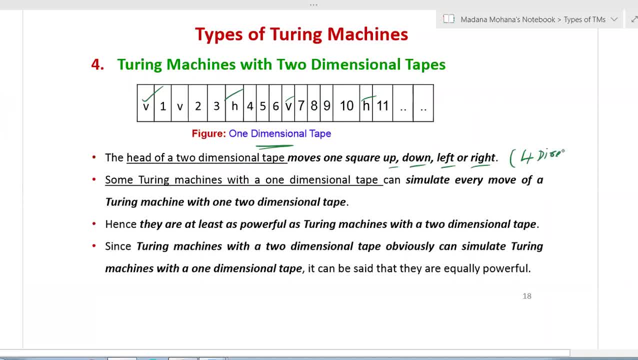 here you can see four directions. in our basic model of turing machine we have only two directions, either left or right. now here extra up, one down, total four directions are there now some turing machines with one dimensional tape can simulate every move of a turing machine with two-dimensional. 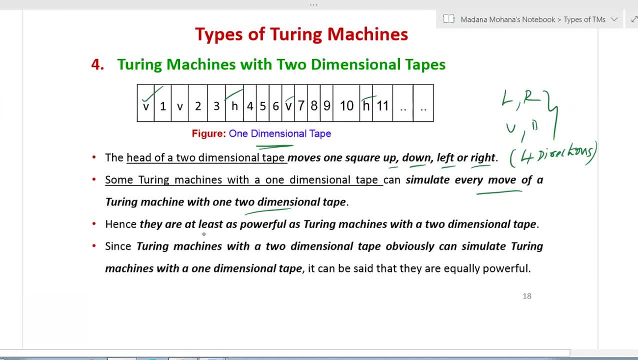 one two-dimensional tape. so hence they are at least as powerful as the turing machines with the two-dimensional tape. then turing machines with a two-dimensional tape obviously can simulate turing machine with one-dimensional tape. latter depends on the latter. it can be said that they. 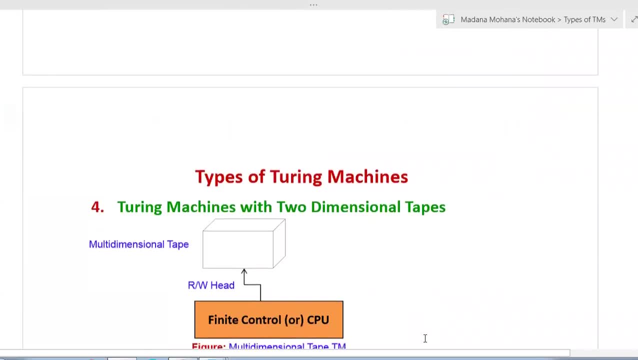 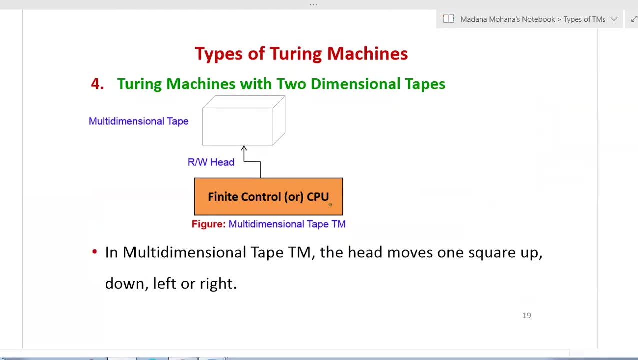 are equally powerful. so now another example of two-dimensional tape. here you can see that the tape is represented in the form of a cubicle. more than two-dimensional, now, this is multi-dimensional tape example, which contains one reader, right header. so in multi-dimensional tape turing machine the head moves one square up, one square down, one square left or one square. 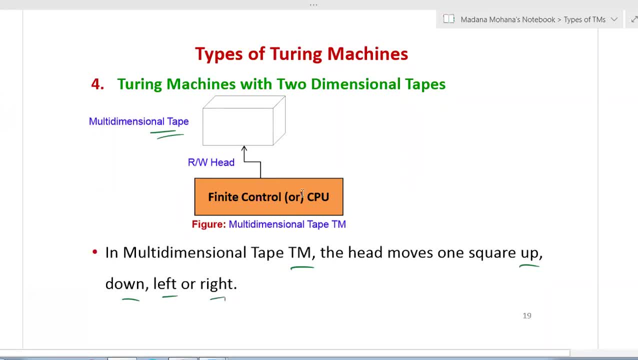 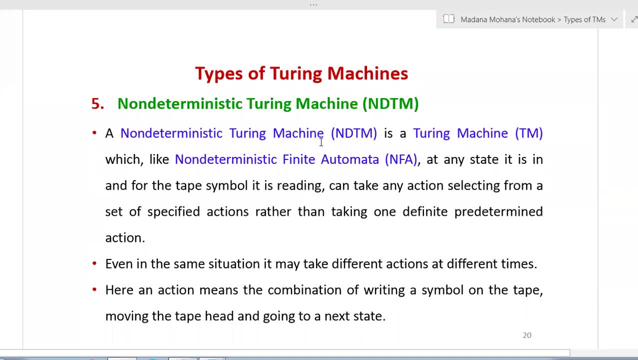 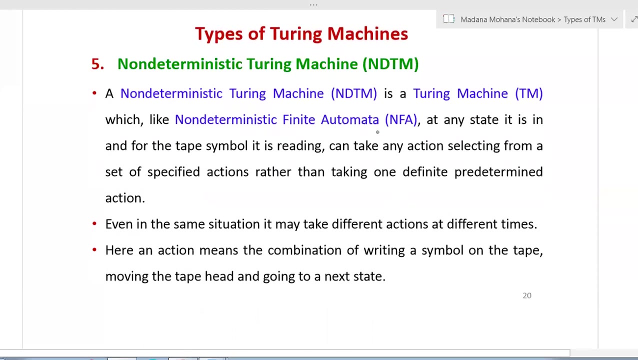 right. all four directions so are possible in multi-dimensional turing machine. then, coming to the last type of turing machine, non-deterministic turing machine, so which is looks like non-deterministic finite automaton in non-deterministic finite automaton from a state on one input. 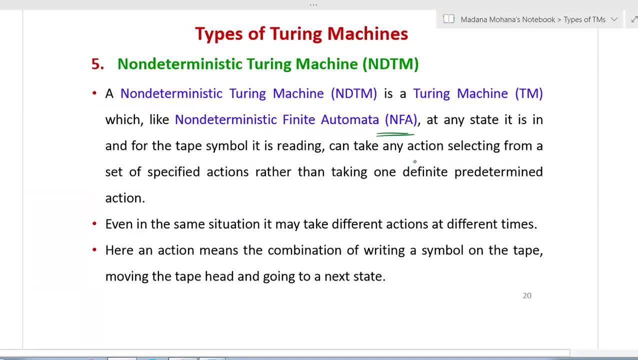 it will be in several next states with the same input. that is possible in non-deterministic and even with empty string, that is, with nuller. so it moves. so these are all allowed in nuller, non-deterministic, finite, automaton, whereas deterministic these are all not allowed. so this: 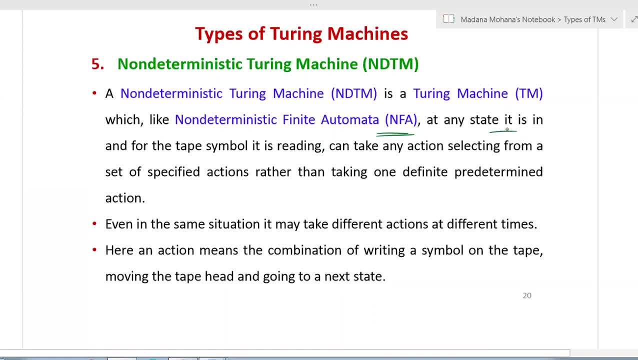 looks like non-deterministic finite automaton, at any state it is in and for the tape symbol it is reading, can take any action, selecting from a set of specified actions rather than taking one definite, pre-determined. that's why it is non-deterministic, even in the same situation. 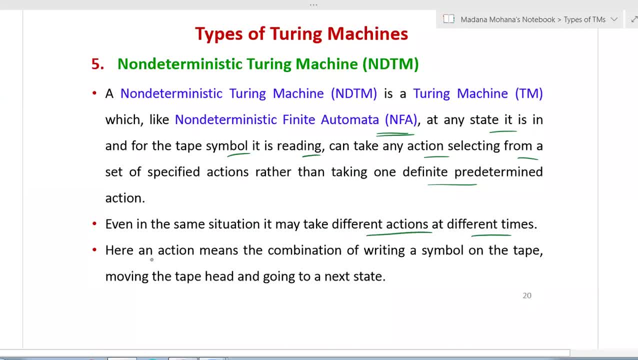 it may take different actions at different times. here an action means the combination of writing a symbol on the tape, moving the tape head and going to the next state, like transitions. so for example, here from a state on a tape symbol. so several possibilities, several next moves. that's what this is. 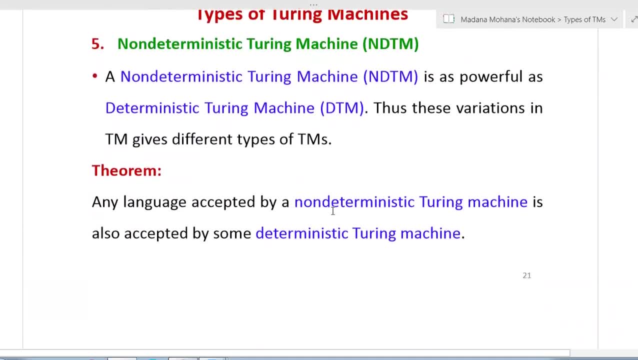 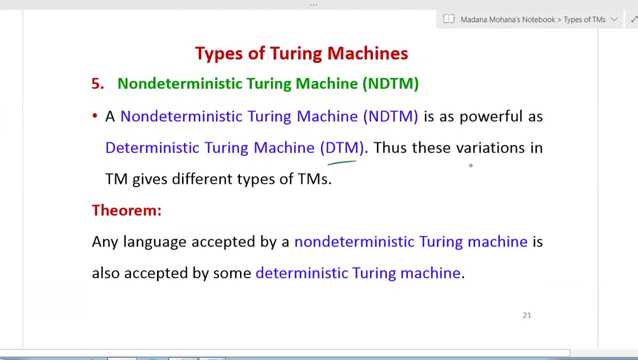 so let's examine this again. on the gates 돼요: nondeterminism. so now, a non-deterministic turing mission is as powerful as deterministic turing mission. does these variations in turing missions use various types of turing mission? now there is one theorem related to this nondeterministic turing mission: any language accepted by a 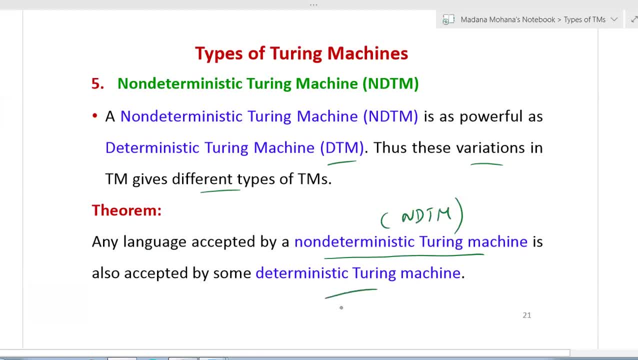 nondeterministic turing mission which is also accepted by some deterministic turing mission. not all deterministic turing missions are able to accept deterministic turing missions may not be turing machine some deterministic turing machine. this is the theorem equivalence of non-deterministic 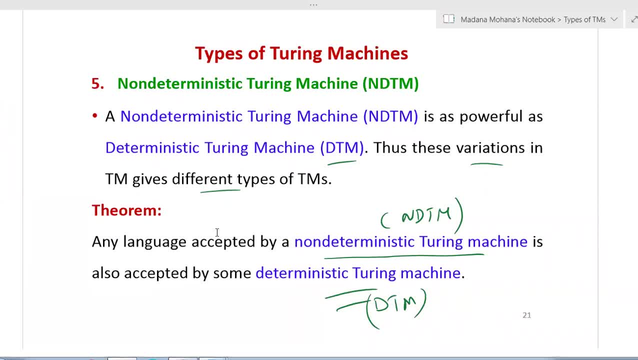 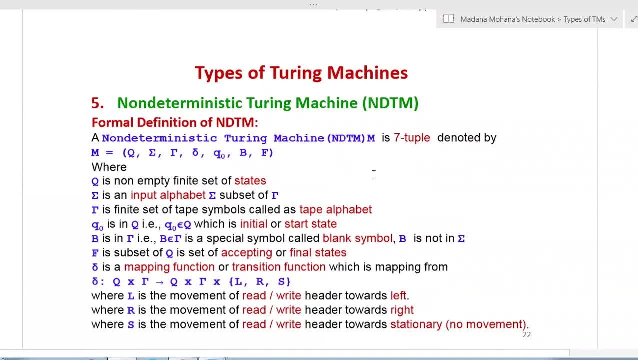 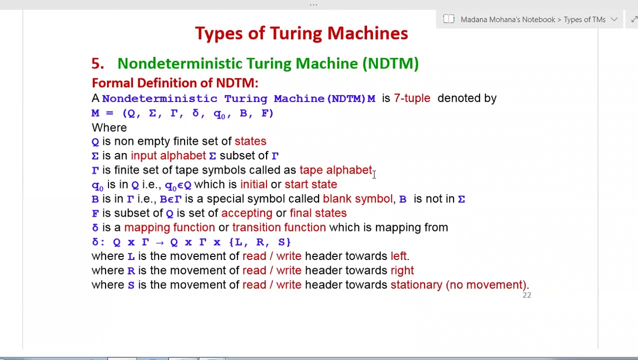 to deterministic. but here we don't have the conversion procedures for non-deterministic to deterministic, like non-deterministic finite automata to deterministic finite automata. then coming to the formal definition of non-deterministic turing machine, which is same as turing machine, here the only difference you can observe while defining delta, there only. 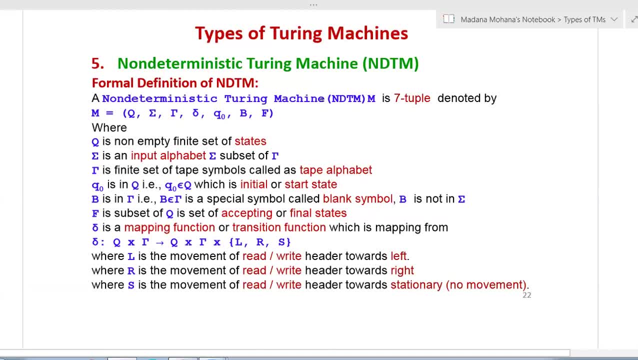 it changes, remaining all are same. so a non-deterministic turing machine. m is a seven-tuple denoted by m, equal to q, sigma, tau, delta, q naught, blank, f, where q is non-empty set of states, sigma is input alphabet, then tau is tape alphabet, then q naught is initial or start state. 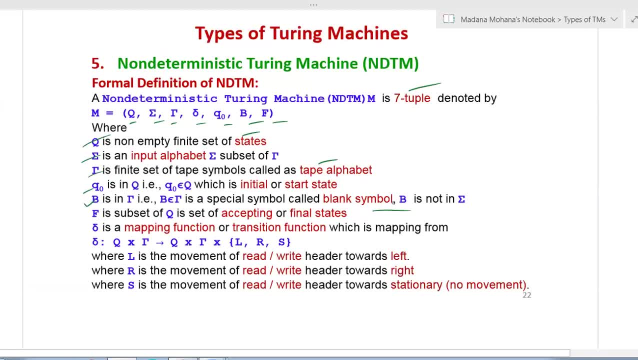 then v is in tau, which is a blank symbol, then f is a subset of q, that is set of accepting our final states. then delta is mapping function or transitive function. so which is mapping? from here you can see the difference: q cross tau, two, q cross tau. 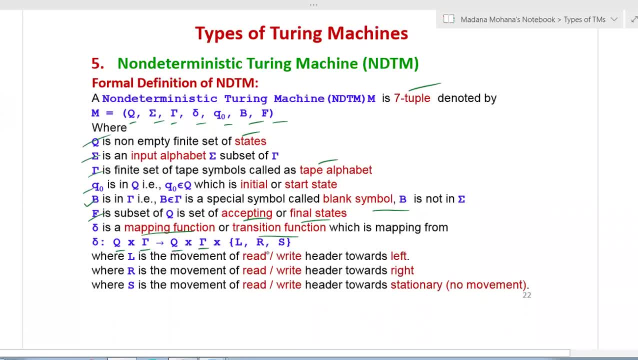 cross l comma r in normal turing mission. but here one more extra direction is added. that is yes. here s is the movement of reader right header towards stationary. that means no movement, stable, whereas l means, as usual, movement of the read right header towards left, then the movement of reader right header towards right. that is the difference here in the mapping. 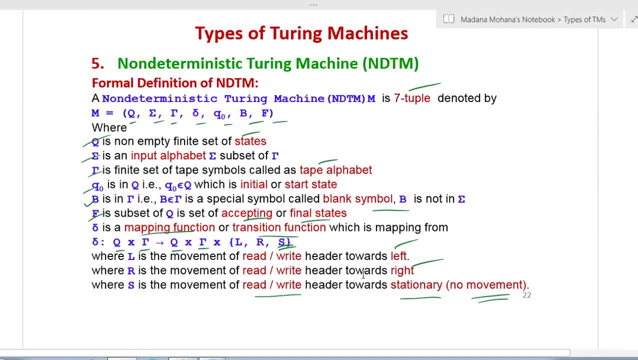 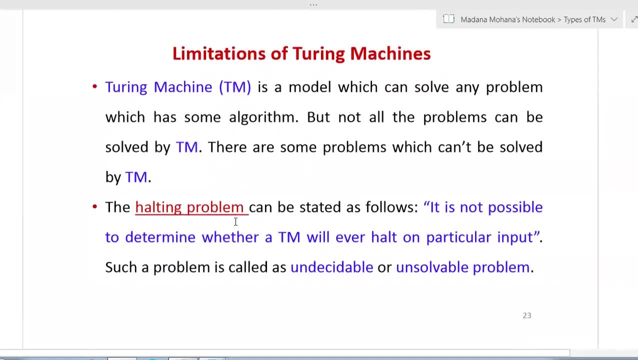 so one more direction is added, that is stationary, denoted by yes, remaining all are same as our basic turing mission. then there are some limitations of turing missions. so turing mission is a model which can solve any problem, which has some algorithm, but not all the problems can be solved by the turing. 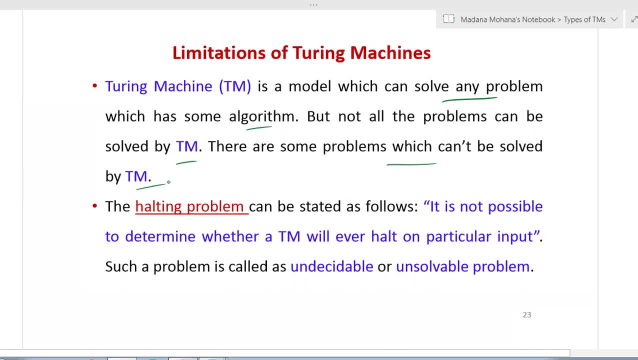 mission. so there are some problems which cannot be solved by a turing mission, which are called as undecidable problems. so one of such examples is the mission function. example is the halting problem can be stated as follows: The statement of Turing mission- halting problem: See. sometimes you will get a question on this. explain about the Turing. 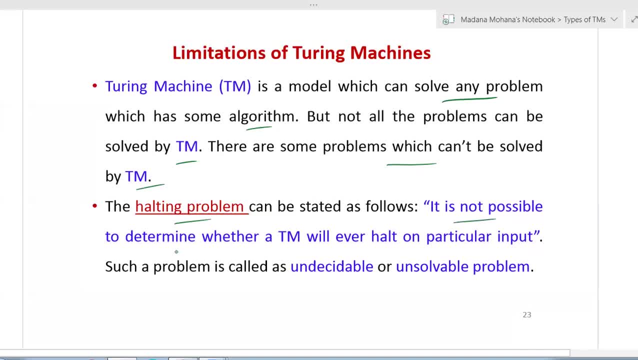 mission halting problem. So the statement is: it is not possible to determine whether a Turing mission will ever halt on particular input. That means on all inputs. it cannot be halted. So such a problem is called as undecidable or unsolvable problem. So therefore, 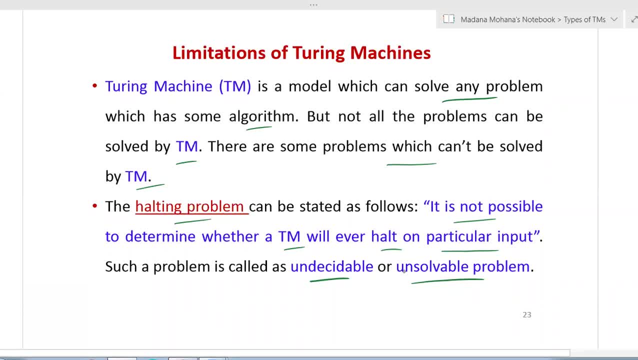 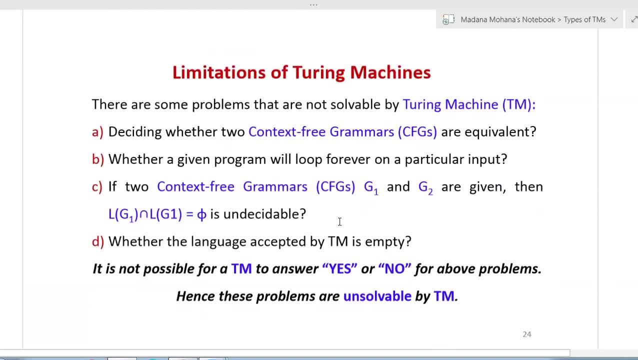 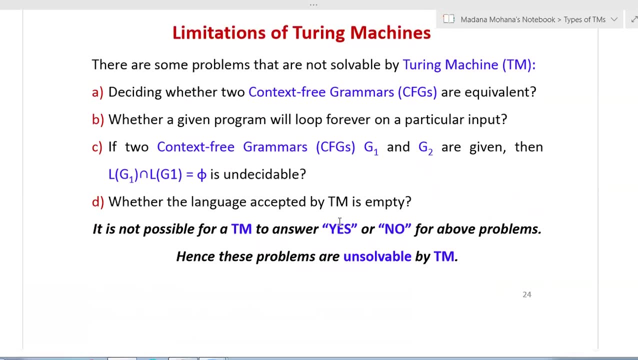 the Turing mission halting problem is undecidable or unsolvable. So this is the statement of Turing mission halting problem, Then other limitations. There are some problems that are not solvable by Turing mission, So which are called as: what are the problems that can't? 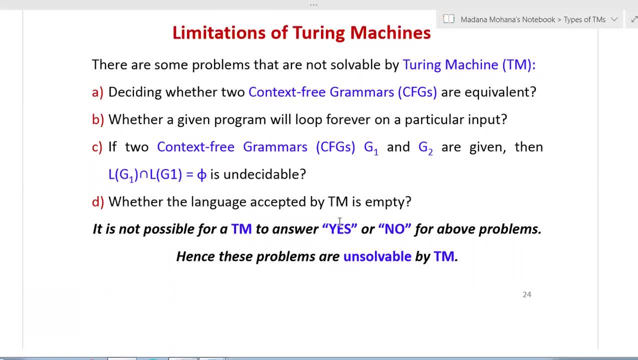 be solved with a Turing mission. that is called as unsolvable or undecidable problem about Turing mission. So the following are some of the problems which are not solvable by the Turing mission, So those are called as unsolvable. The first one is deciding whether two context free grammars. 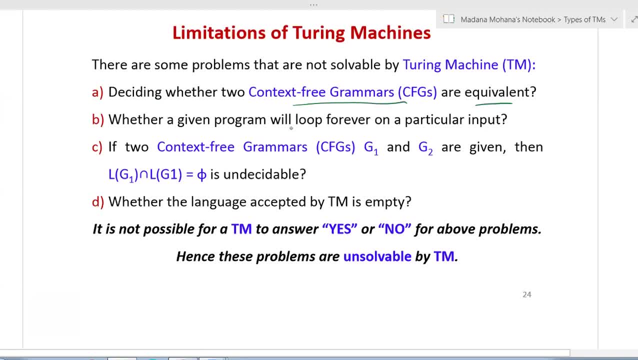 are equivalent. So this is undecidable or unsolvable using Turing mission. All these problems are not solvable with Turing mission, So which are called as undecidable or unsolvable problem. Then the second one: whether a given program, any program, will loop forever on a. 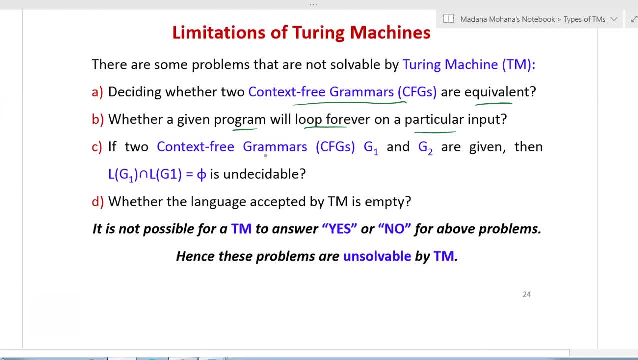 particular input. This is also undecidable. Then if two context free grammars, say G1 and G2, are given, Then the intersection of these two context free grammars is undecidable. Then the intersection of these two context free grammars is empty. So L of G1 intersection. 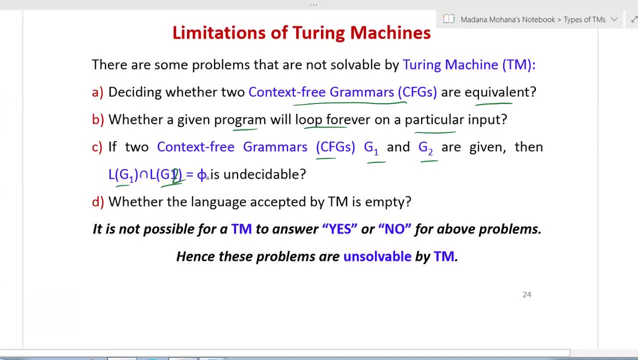 L of this is G2.. L of G1 intersection, L of G2 equal to pi. This is also undecidable. We can't determine- Then the fourth one- whether the language accepted by Turing mission is empty. This is also unsolvable or undecidable. So these are some of the problems related. 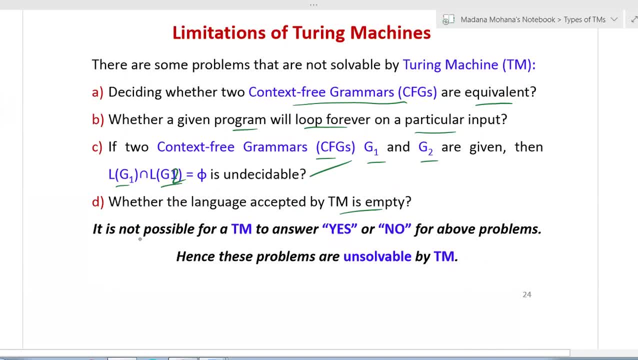 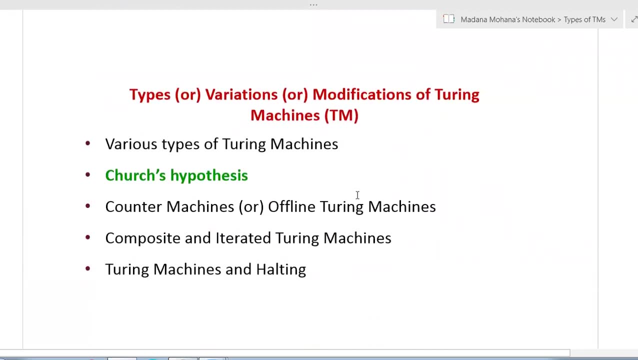 to Turing mission which are unsolvable or undecidable. So here it is not possible for a Turing mission to answer yes or no For above problems. So hence these problems are unsolvable by Turing mission. These are all some of the limitations of Turing mission. Then coming to our next variation in Turing, 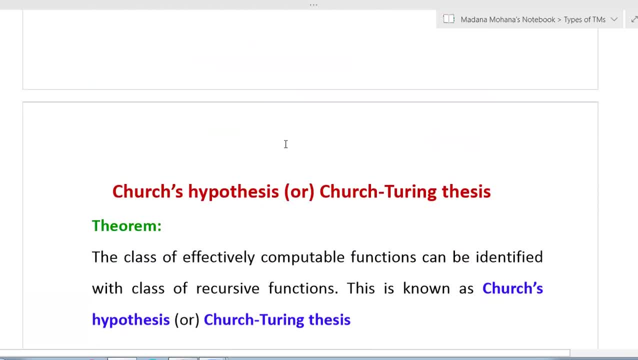 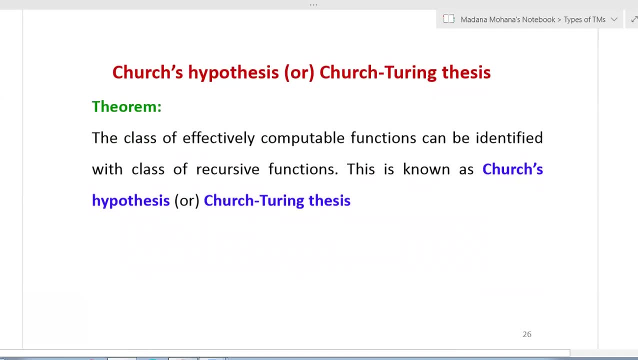 mission, Chet's hypothesis, also called as Chet's Turing thesis. So this is one approach related to Turing mission. A statement of this approach is which is called as theorem, The class of effectively computable functions. So we have one set of classes in the class. 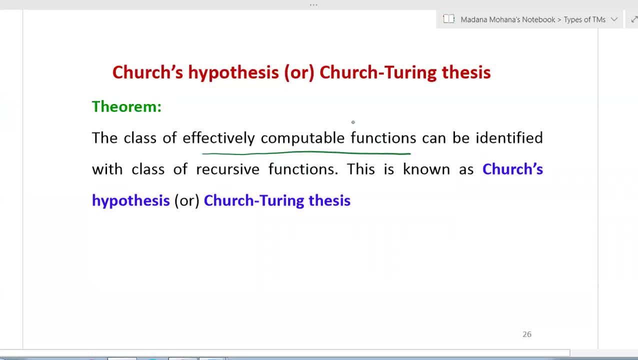 class which are effectively computing using computable functions, So can be identified with the class of recursive functions. This is known as Church hypothesis or Church Turing thesis, So any function that is being computed by a Turing machine is called as computable function. After this concept, we will discuss about computable functions, then construction. 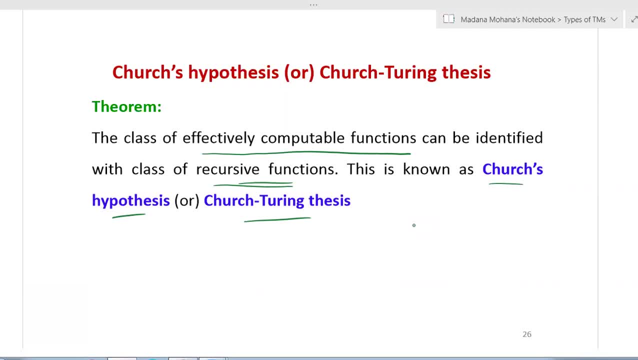 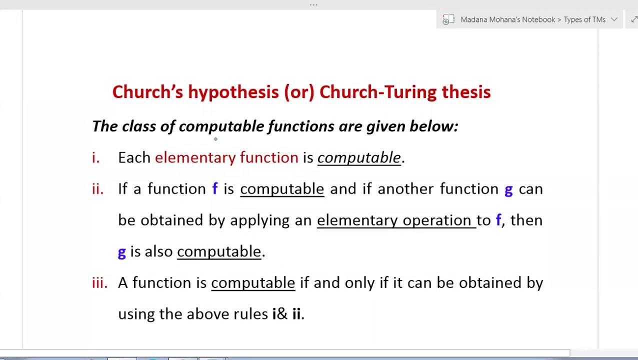 of Turing machine for computable functions, Any function that is being constructed by a Turing machine, so then that is called as computable function. So those can be identified with class of recursive functions. This approach is called as Church hypothesis or Church Turing thesis. So now, here you can see what are the class of computable functions. So the class: 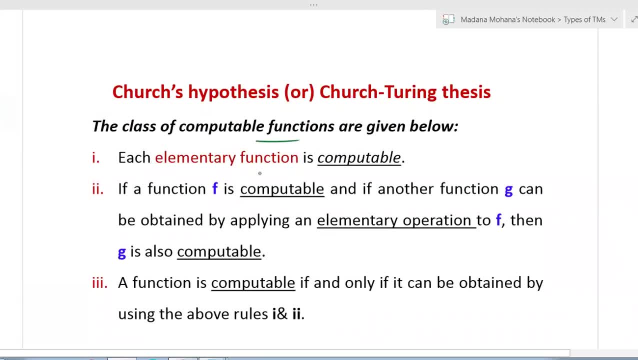 of computable functions are given below. You can take any elementary function which is computable. Each elementary function, a basic function, is a computable. then if a function f is computable and if another function, g, can be obtained by applying an elementary operations to f, 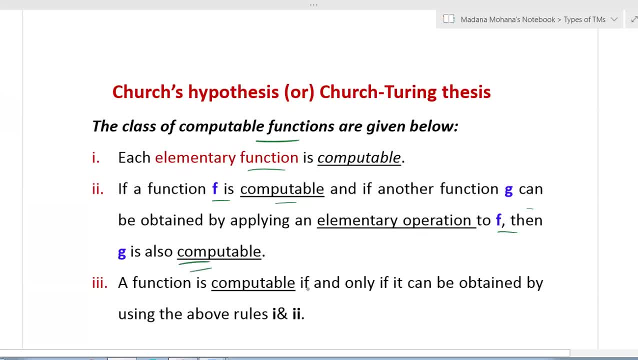 then g is also computable, Then a function is computable if, and only if, it can be obtained by using the above rules 1 and 2.. So this definition is some what similar to recursive definition of regular expressions. So, regular expressions, we have defined some. 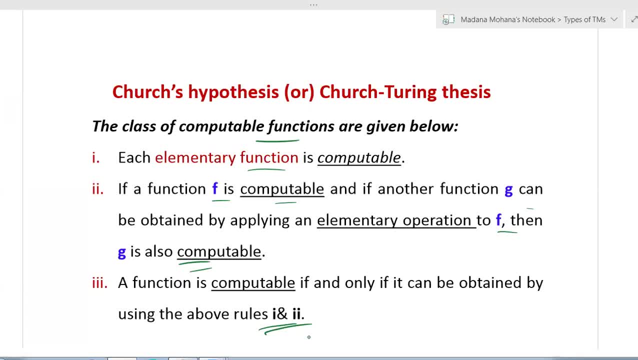 set of rules, rules. then by repeating all the rules by once or several times, what are the applications you will get? those are all only the regular expression, like the class of computable functions. also here two rules are given. each elementary function is computable. then if a function 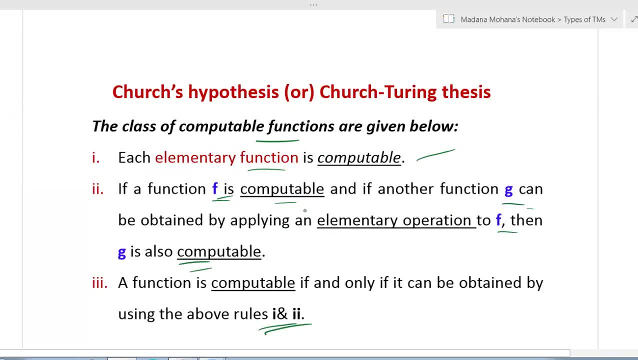 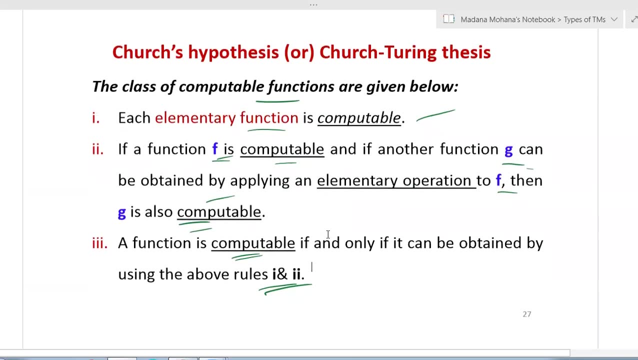 f is computable, and if another function, g, can be obtained by applying an elementary operation to f, then g is also computable. then by repeating the above rules, one and two, whatever the results we obtain, those are all only computable. these are all the class of computable functions. 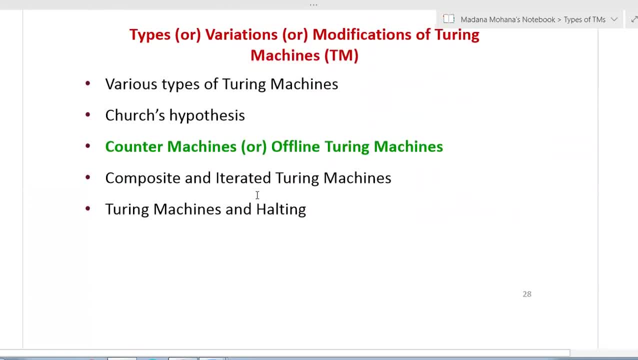 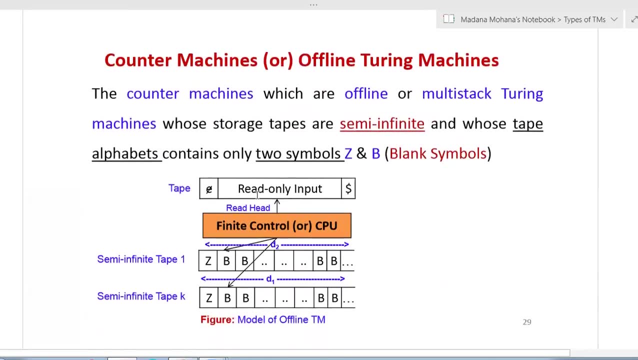 so then, coming to our next variation of turing mission: counter mission or offline turing mission. so this is also one kind of turing mission, actually. so now, what is counter mission or offline turing mission, which is also called as a multi-stack turing mission? here you can. 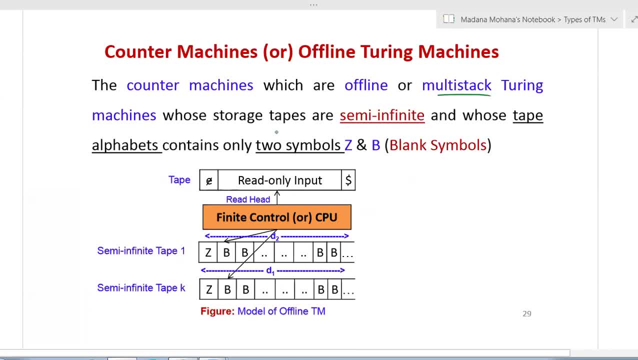 see the name itself gives multi-stack turing mission. now here the counter missions, which are offline turing mission or multi-stack turing missions, whose storage steps are semi-infinite, not fully infinite, semi-infinite, and whose type alphabets contains only two special symbols called as z and b, which are called as blank and initial. 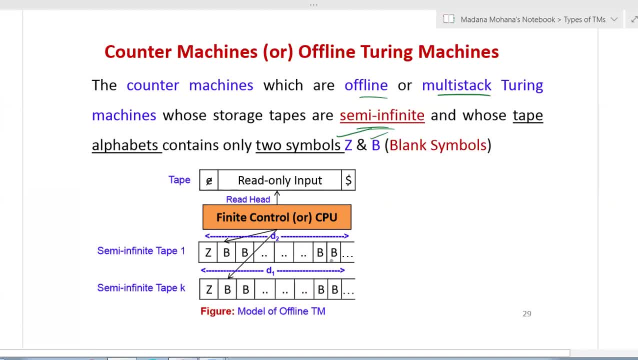 symbol. now you can see the model of offline or counter mission or multi-stack turing mission which consisting of one finite control. then we can see the machine is somewhat similar to multi-tape turing mission. more than one tape is there, but in multi tape so one is fixed tape. here you can see the primary tape which 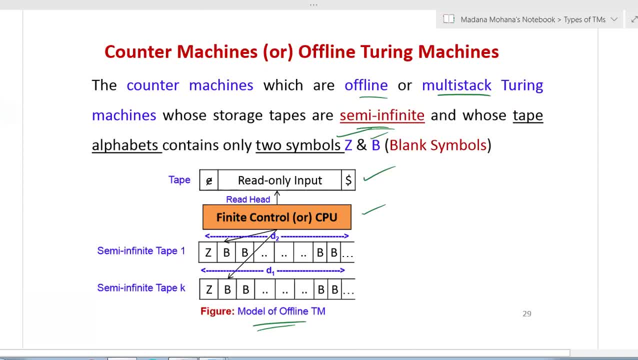 can be represented on top. so it is restricted with finite length by including two end markers, that is, one is at left end, another one is at right end. then in between we have the input. the input only you can read, we can't write. so that's why it contains only read, only input. 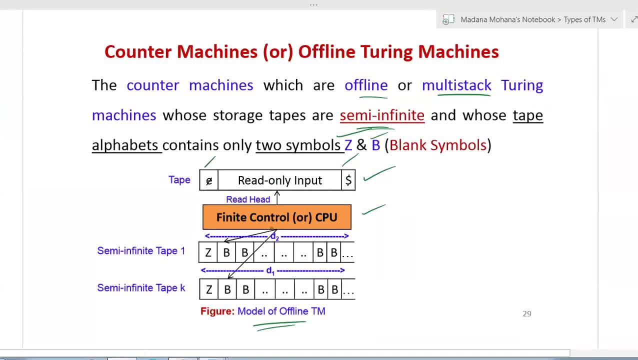 this is a finite tape, then other tapes represented on the bottom of the finite control. so here we have semi-infinite tape one and the semi-infinite tape two and so on. semi-infinite tape k. here you can see why you are calling it a semi-infinite. the left hand is fixed, then right hand is open. 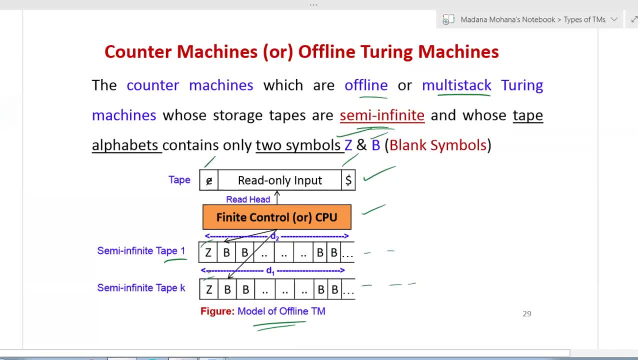 extended infinitely. so now these tapes, lengths are denoted by uh like d1, that is a distance, then d2 for a particular tape like. so all these semi-infinite tapes, uh, left cell, consisting of z, that is the initial symbol, then all are filled with blank symbols. now let us see some functionality. 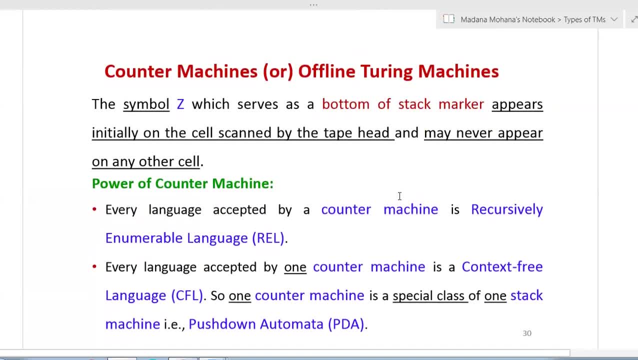 about this type of turing mission or counter mission or offline turing mission. the symbol z, which serves as bottom of stack marker- so here we will use the concept of stack, that is pde, so appears initially on the cell scanner by the tape head and may never appear on any other cell. z appears only. 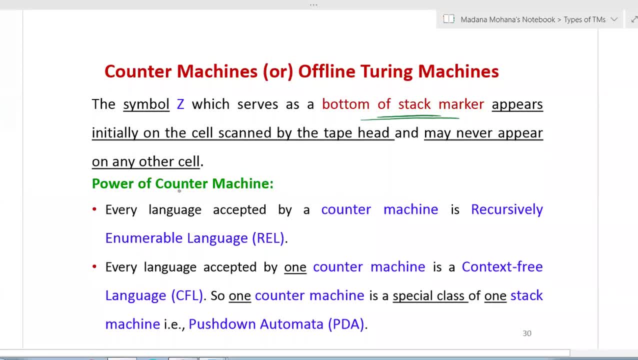 in one cell. so initially then power of the compute, counter mission power, or the importance of counter mission. so every language accepted by a counter mission which is called as recursively enumerable language. so if we have a counter mission, turing mission, if any language that is accepted by this, 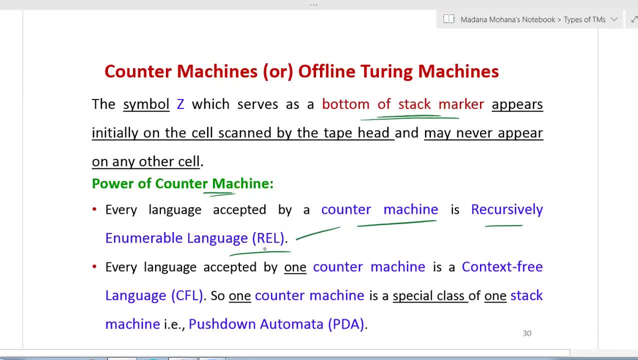 counter mission, then the language is called as recursively enumerable language. then every language accepted by one counter mission so is a context free language with only one counter mission. so one counter mission is a special class of one stack mission. so that is pushdown automaton. so if 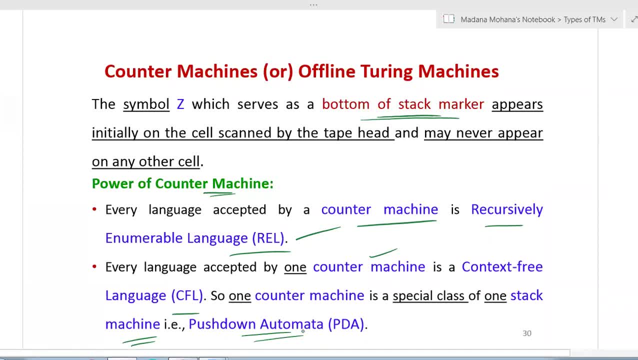 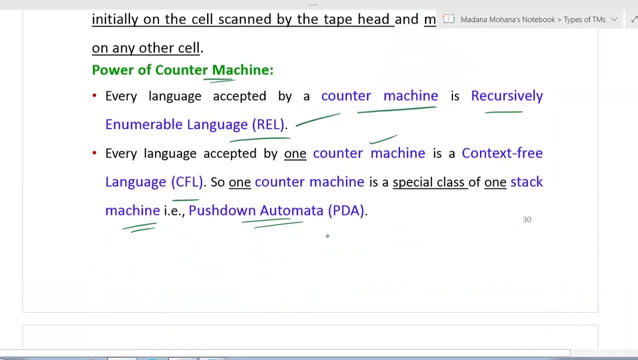 any language accepted with only single counter mission, then that language is called as context free language. then this is the special case of one stack mission that is pushdown automaton. then you running your system based on the description down. if they are not validif you're required to. 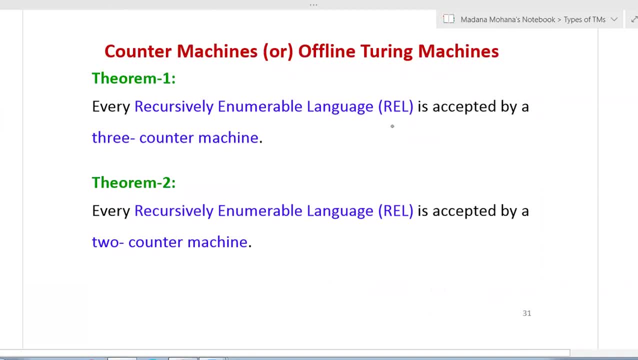 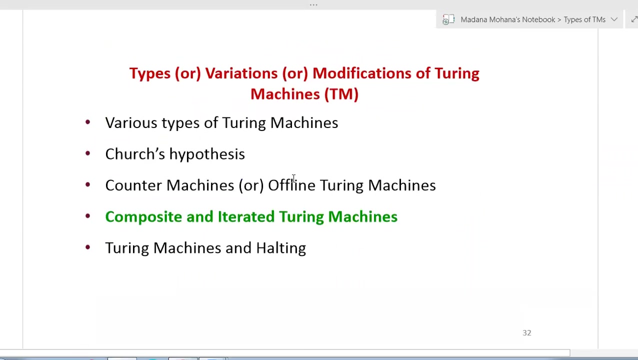 make permissions to use the print function in a way that we're not trying to find the gado understand quê to other variation or modification of Turing mission: composite and iterated Turing mission. So composite is nothing but a hybrid type combination. Iterated means repetitions, So 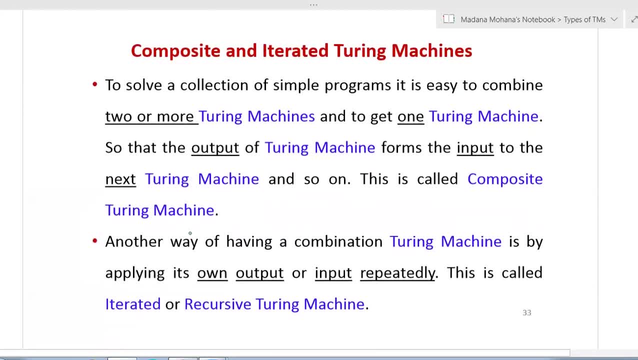 then how to define these two? To solve a collection of simple programs, it is easy to combine two or more Turing missions. by combining two or more Turing missions and get one single Turing mission, So that output of Turing mission forms the input to the next Turing mission. 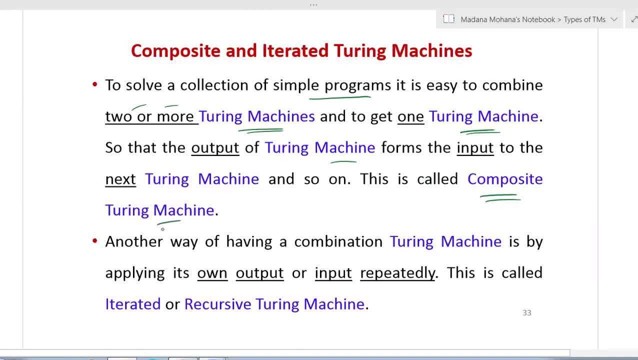 and so on. This is called as composite Turing mission. That means one Turing mission output will be considered as input to the next Turing mission, then next Turing mission output should be considered as the input of next Turing mission, and so on. Then combining all these, 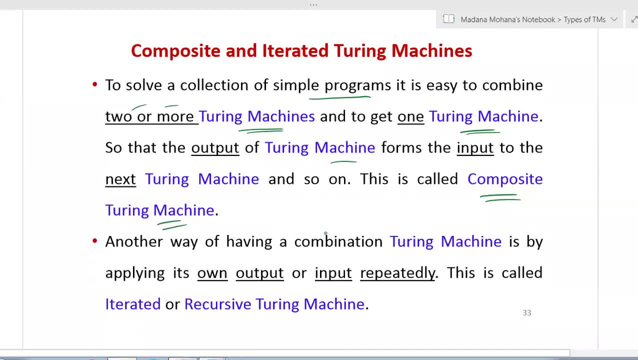 So we will get the single output that is called as composite Turing mission. Then another way of having component Turing mission is, in other words, the Kart 이런 geworden creatingял 이ии. combination Turing mission is by applying its own output or input repeatedly a particular 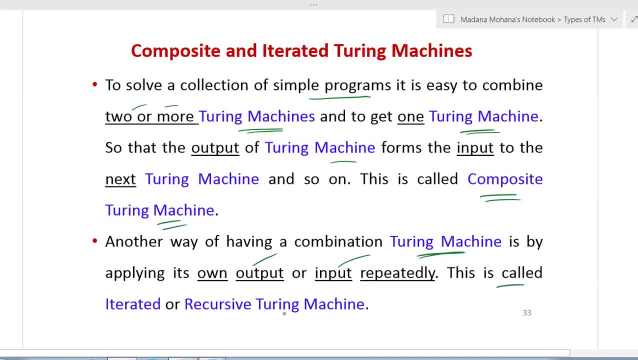 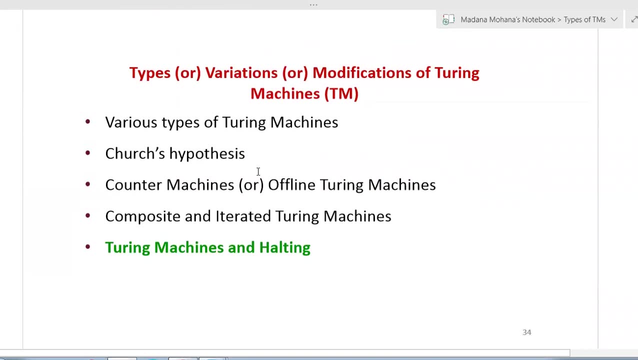 Turing mission input or output that can be repeated, then this is called as the iterated or recursive Turing mission. so these are all the two more variations of Turing mission: composite and iterated Turing mission. that's all about this one. it's very simple. then the last variation of Turing mission is Turing missions and halting. so here we already discussed. 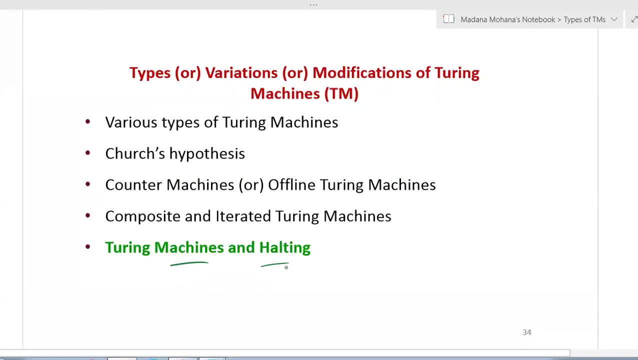 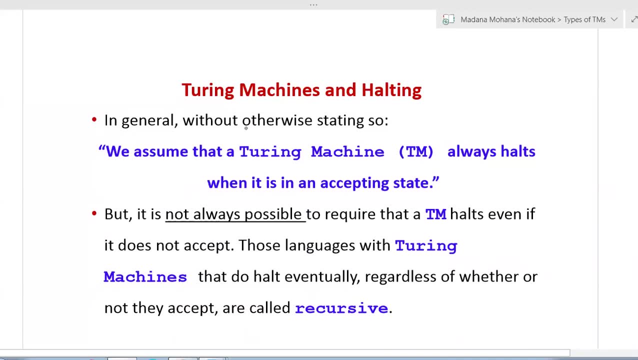 the statement of halting problem of Turing mission. so here we will focus more on that. so now here, Turing mission and halting in general, without otherwise stating so, the following statement: we assume that a Turing mission always halts when it is in accepting state. so this is proven statement. so whenever the Turing mission is in accepting state, compulsory. 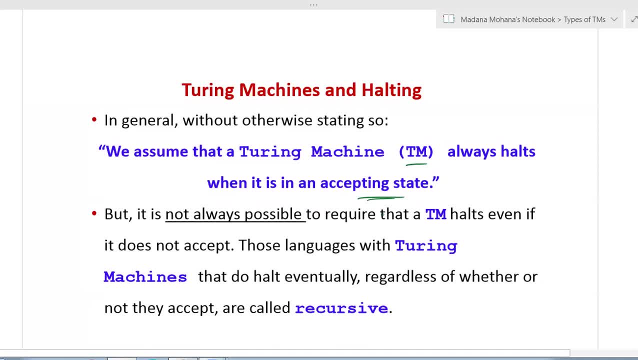 the Turing mission is in accepting state, compulsory every time it halts if it is not in accepting state. so there may be chances with less possibilities, but it is not always possible to require that a Turing mission halts even if it does not accept. so those languages with Turing missions that do halt eventually, regardless of 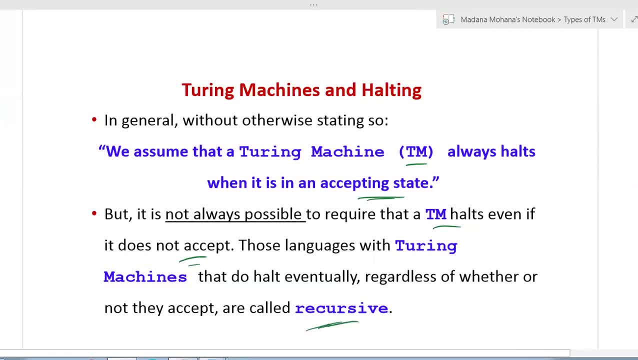 whether or not they accept, are called recursive. see, here we discussed the two languages. one is recursive and recursively enumerable languages. so recursive languages, which gives the both results, that is yes or no, both results, then that is fully decidable. whereas recursively enumerable languages, which gives only the result, is yes, irrespective of any input. 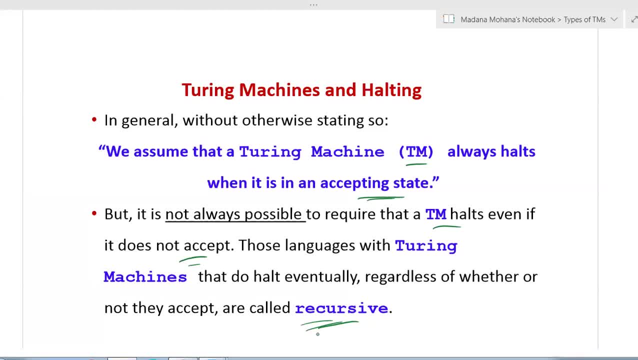 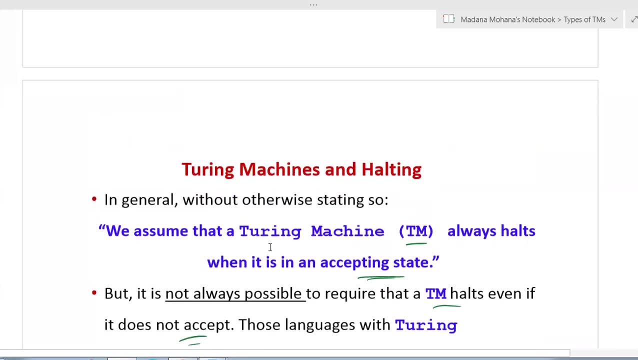 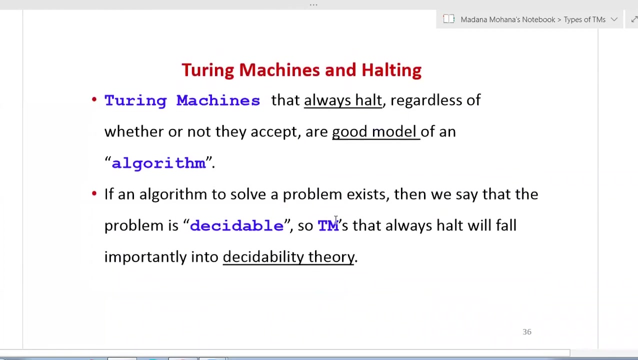 then this is semi decidable. so that's why Turing mission halting may be possible means it satisfies the concept of recursive language. So for every input it halts, even for recursive enumerable, only for some, not for all inputs or strings. that is the difference between recursive and recursive enumerable language. 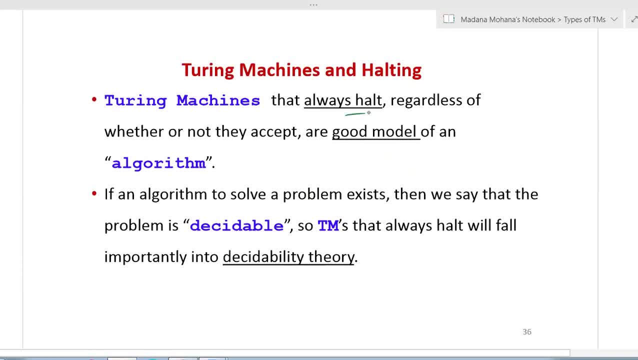 So now same concept is used here: Turing machines that always halt, regardless of whether or not they accept or good model of an algorithm. that means: whenever there is an algorithm, means the problem can be solved, means solvable. if an algorithm to solve a problem exists, then we say that the problem is said to be decidable or solvable. 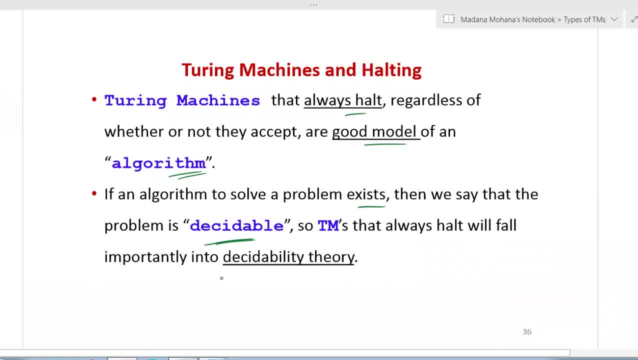 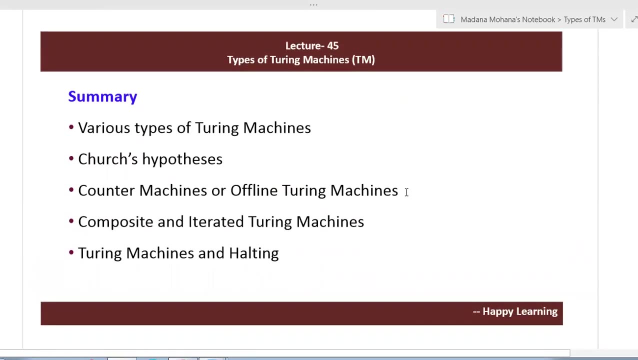 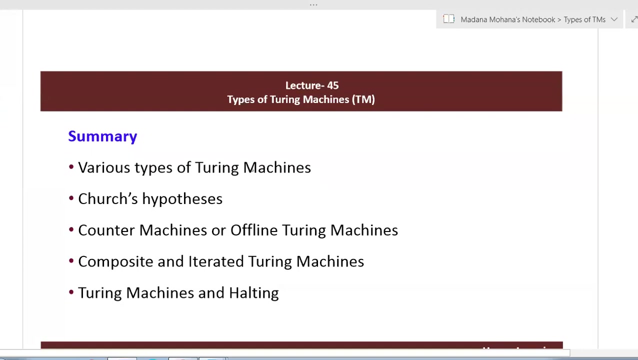 So Turing machines that always halt will fall, importantly, into decidability theory. always halts that means a decidable, solvable, but only some cases. it also means that falls under undecidability theory. Okay, Now let us see- Let us come to summary of this lecture- what we discuss here. we covered first various types. 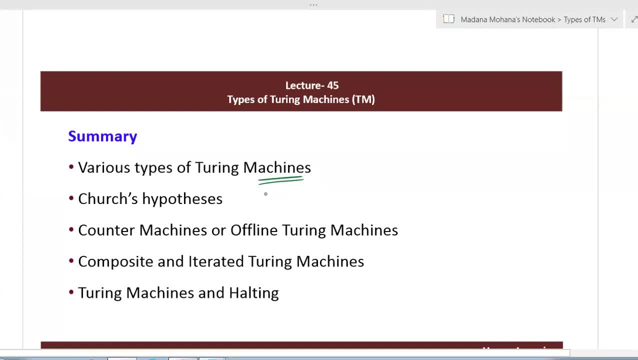 of Turing missions or classifications or categorizations, then other variations or modifications. we discussed about the Church hypothesis or Church Turing thesis. then another variation, counter mission or offline Turing mission, also called as multi-stack Turing mission, then composite and iterated Turing missions and finally Turing mission and halting.